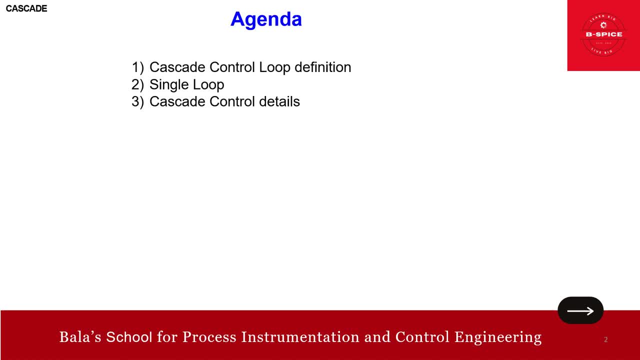 Then we focus on the cascade control details. Okay, primary and secondary loops in cascade control. which is primary and what is a secondary? Okay then, very important, when to use cascade control. Okay, when should cascade control be used- Just remember the meaning, friend: when to use cascade control. When should cascade control be? 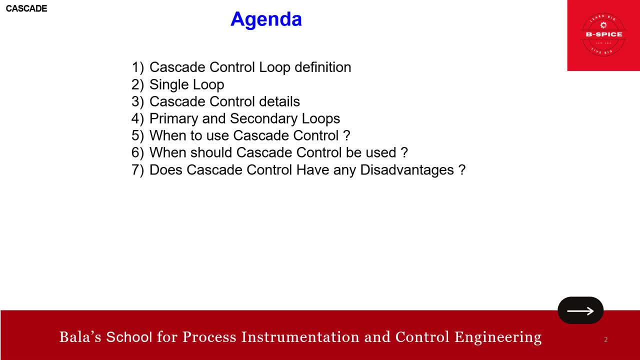 used? Okay. does cascade control have any disadvantage? Yes, let us see what is there. Yeah, when should cascade control not be used? So that is, also, we need to learn. When should cascade controls to be tuned? Okay, tuning. Then finally, the configuration of. 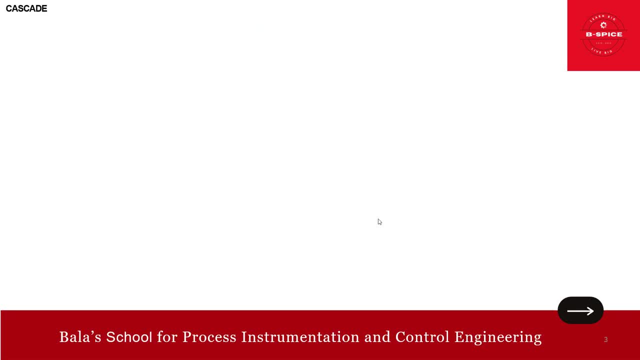 cascade using Yokogawa DC. So these are the points we are going to cover. Okay, friends, good to go. Okay, cascade control loop. As we know, in cascade control loop, two controllers are used. What for? To manipulate a single final control element. That is important. 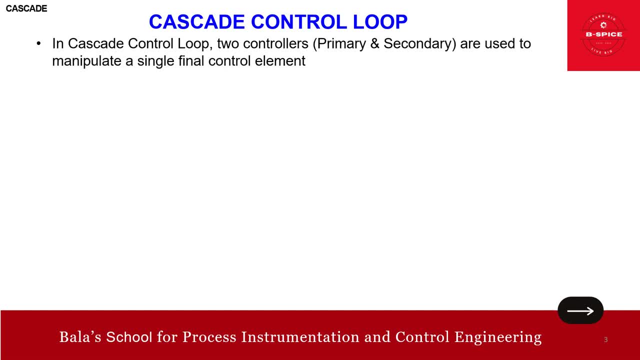 Remember, friends, in cascade loop, two controllers- that is, one is primary, other is secondary- Are used to manipulate a single final element: control element. That is the point, very important. Okay, cascade control uses the output of the primary controller, So that is the another. 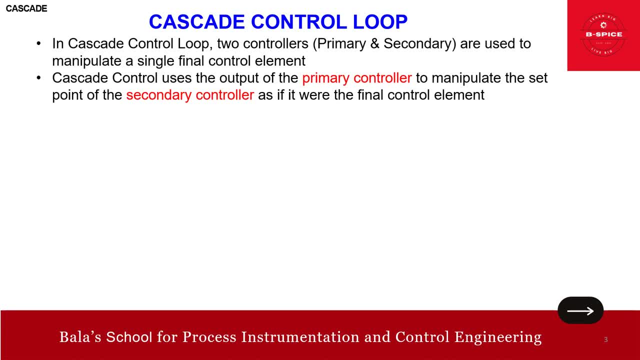 aspect here Very important. Okay, cascade control uses the output of the primary controller. What for? To manipulate the set point of the secondary controller. Okay, you got it right. So cascade control uses the output of primary controller To manipulate the set point of the secondary controller as if it were the final control. 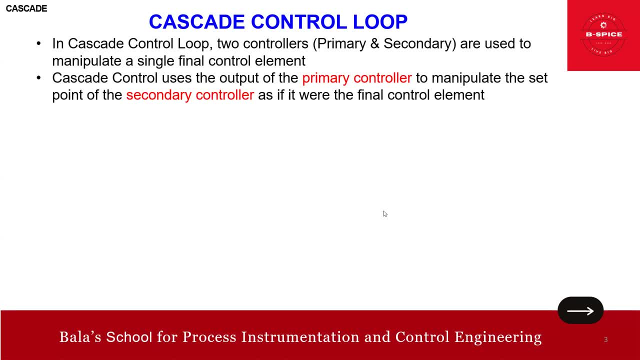 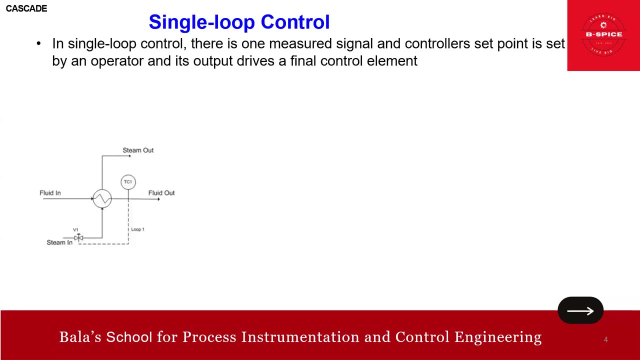 element. Okay, friends, So this is the gist of cascade control loop. I hope you are very clear on this. Of course, experienced engineers know that this is more target for pressures and intermediates. Okay, good to go. Right Now we will see the single loop control. Okay, So, 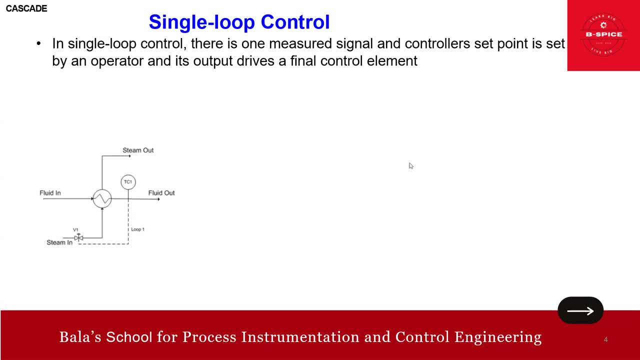 typical example you can see: See, in a single loop there is only one measured variable. Okay, only one measured variable. Okay, then you can see: the controller set point is set by an operator. Okay, is set by an operator, and the output drives the final control element. Okay, here, right. 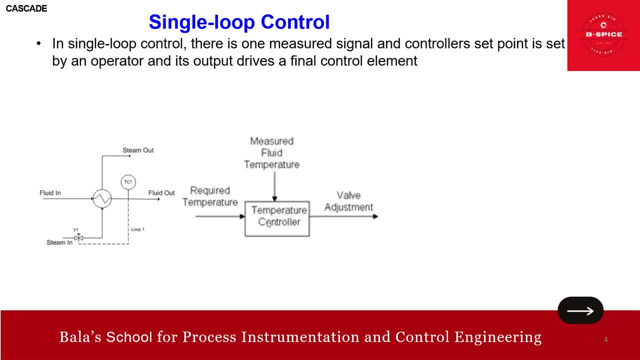 friends, Right? So this is a typical example Like, for example: see the required temperature. this is your controller. this is your valve adjustment. then you have measured fluid temperature. Okay, then this is also a typical single loop control, As you can see here. this is the time the feed is coming in. This is your. 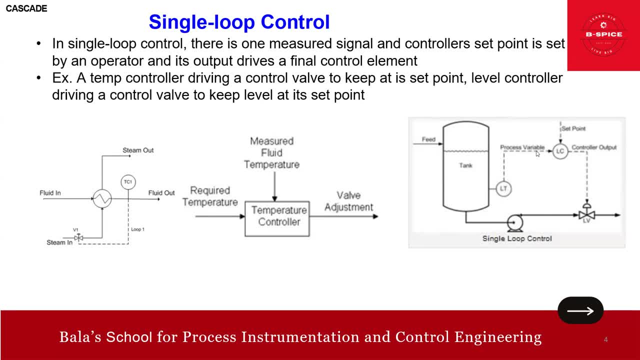 you know, measured process variable. right, This is the LT process variable. then it is controlled using a level controller. This is your output and it's controlling the valve actually. Okay, that's it, friends, A single loop controller. there is only one measured variable. So that is the. 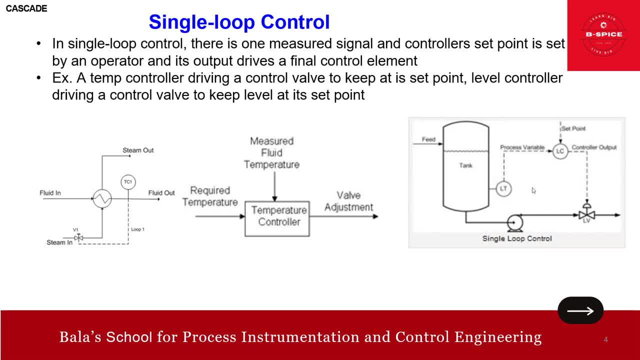 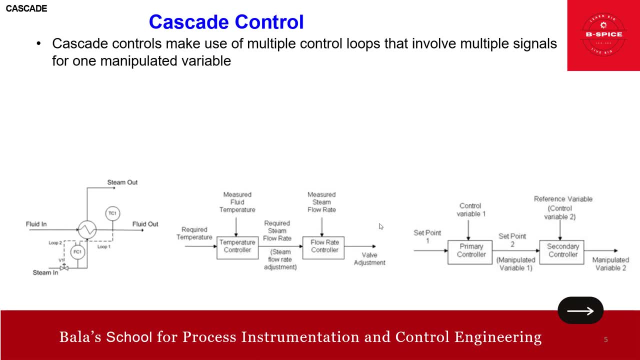 point here. Here it's a temperature, Here it is a level. Okay, so that's a pointer. Okay, now we go to cascade control. So cascade control makes use of multiple controls that involve multiple signals for one manipulated variable. So that is the point: multiple controls. You can see here multiple. 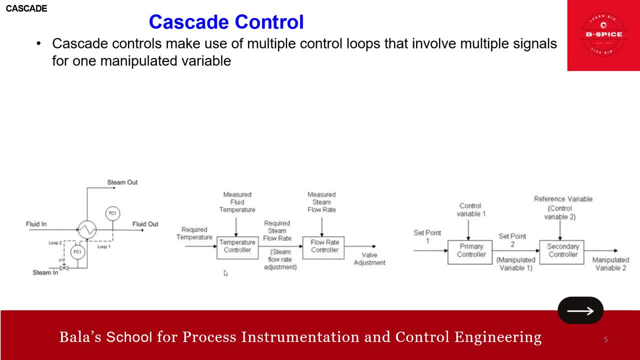 variables. See the temperature here. also, flow is there right Here. temperature, the flow is there right. Yes, that is the point here. So this is a control variable one. this is the control variable two. Yeah, I hope now you got it between the difference between the single and cascade. 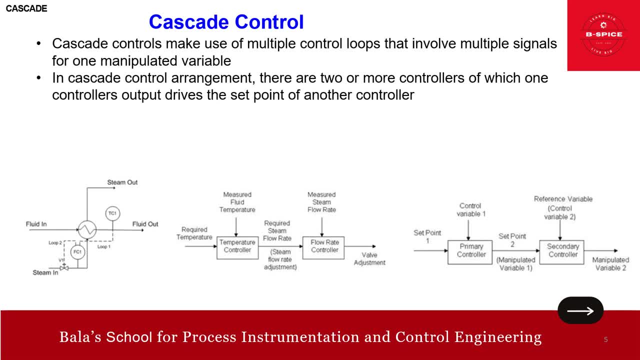 Okay, in a cascade control arrangement there are two or more controllers, Okay, one or two, Okay, of which the controller output drives the set point of another controller. Okay, so this gentleman, actually this- actually drives the set point of another controller. Okay, right, The controller. 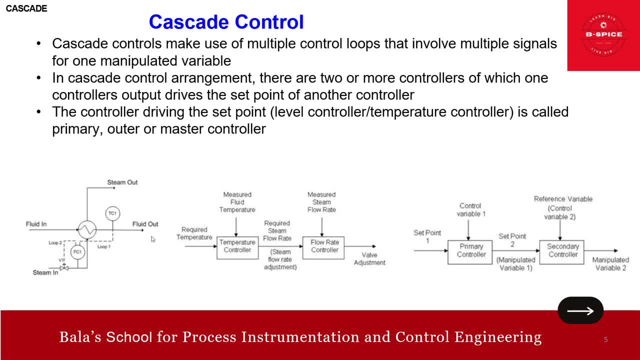 driving the set point, whether it's a level control or flow. temperature control is called the primary. Okay, the controller driving the set point here, which is driving this, is driving the. So in this case, temperature control. this is the primary and we call it as outer or 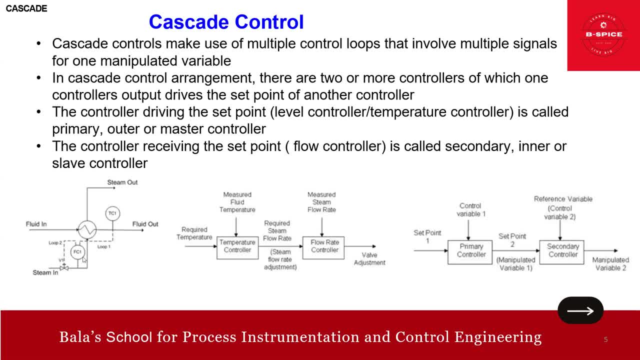 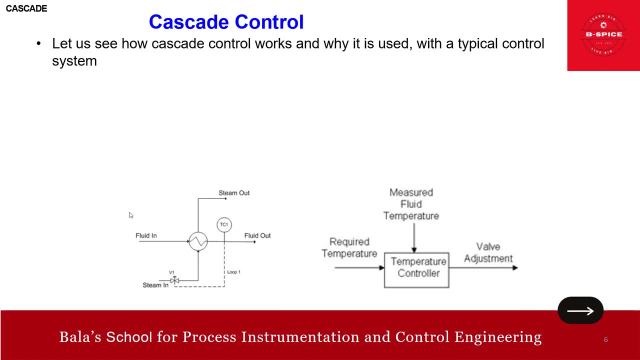 master controller. Okay, Then the controller receiving the set point, in this case flow controller. This is called secondary or inner or slave controller. You got it, friends. Okay, Good to go. So to add on more, let us see how cascade control works and why it is used. with a typical, 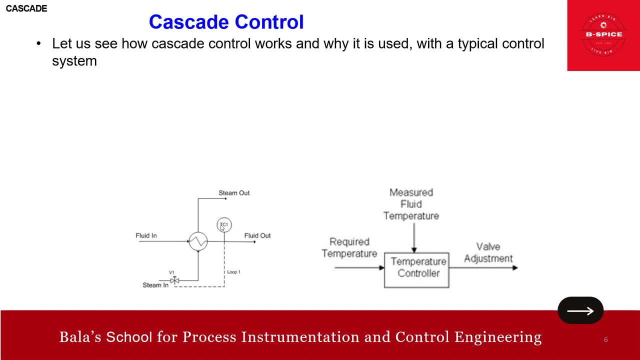 control system. An example. Okay, This is your typical example. Okay, Of course, this is a typical example for what you call a single loop. Yeah, The below control system is the one that used to adjust the amount of steam used to heat. 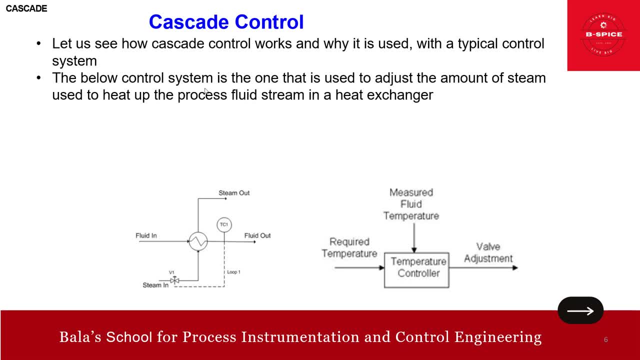 up the process fluid medium in the heat exchanger Right. So this is the one that used to adjust the amount of steam coming in right to heat up the process fluid. This is your fluid in heat up the process fluid in the heat exchanger. 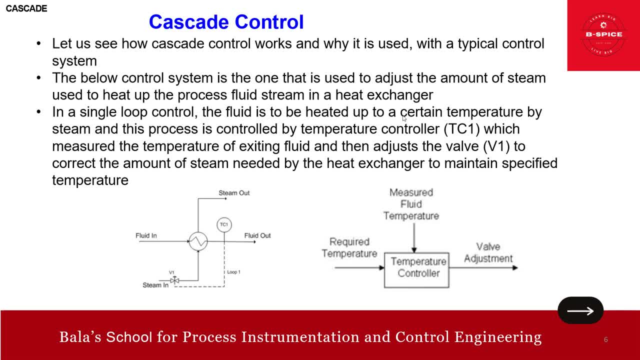 Okay, So in a single loop, the fluid is to heat up the process. fluid in the heat exchanger: Okay, So this is the one that used to be heated up to a certain temperature by steam Right, And this process is controlled by temperature controller TC1, which measure the temperature. 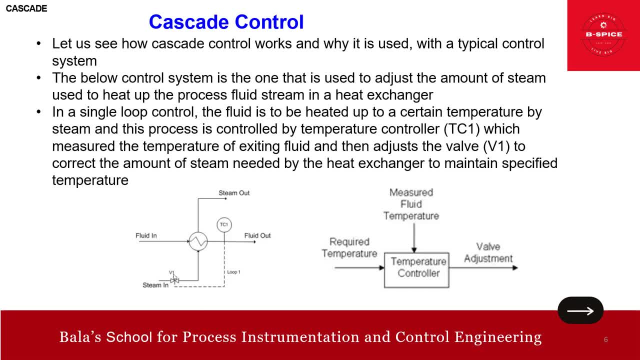 of the exciting fluid and then adjust the valve V1 to correct the amount of steam needed by the heat exchanger to maintain a specific temperature. You got it, friends, Okay. So this one. I just put example actually to, before going in detail to the cascade, just 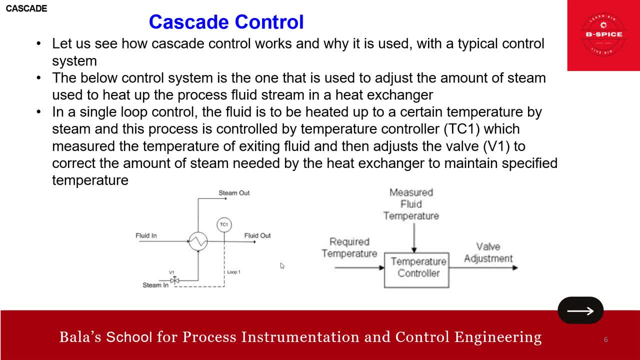 want to put a bit of you know Explanation for the single loop. Okay, Let's move on. So the figure shows here the flow of information from to from the temperature controller. Okay, That's okay. So it works, on assumption that a constant flow of steam is available. 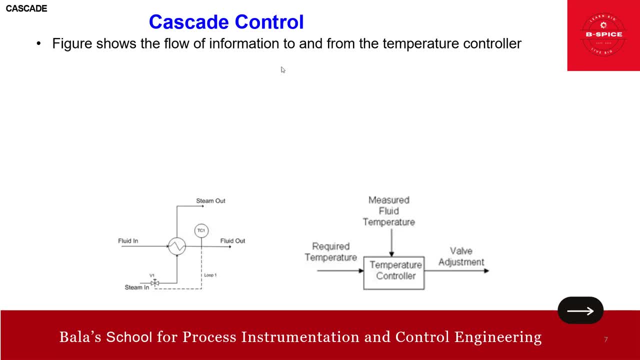 Okay, Here a constant flow of steam is available. So that is the assumption, And the steam to the heat exchanger is solely depend on the opening of the valve. Obvious Right. Yes, Okay, Okay, Okay, Okay Okay. 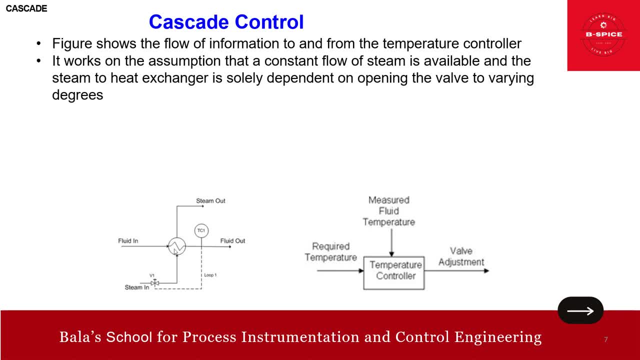 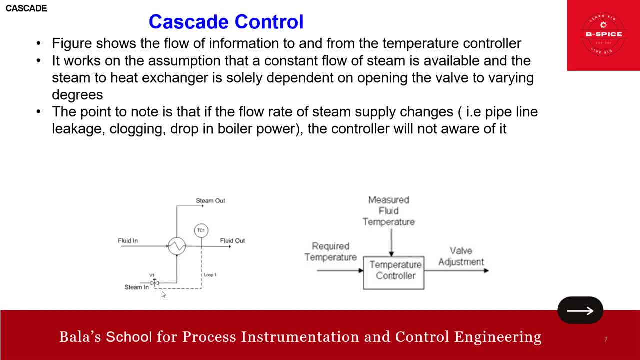 is the point, like how, pipeline leakage, clogging or drop in the boiler power, all these, the controller, this controller will not be aware here What is happening. you will not know. actually Got it. Yes, So the controller opens the valve. this controller opens the valve to the same degree he expecting. 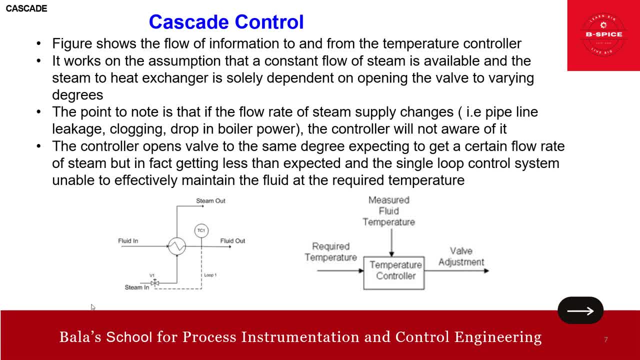 to get a certain flow of steam, rate of steam, but in fact getting a less than expected, and the single loop system is unable to effectively maintain the fluid at the required temperature. so that is the point. you got it, friends. this is the advantage or disadvantage. see the point to note. that is, if the flow rate of the 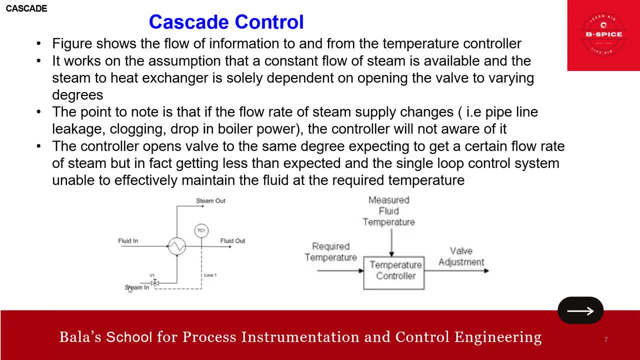 steam supply changes. if there is no change, there is no issue. but if it changes, the controller will not be aware. so what he will do, he will open, he will do the same degree of opening f. okay, so that is the point. okay, so to nullify, to mitigate this only, we are going to use cascade. okay now. 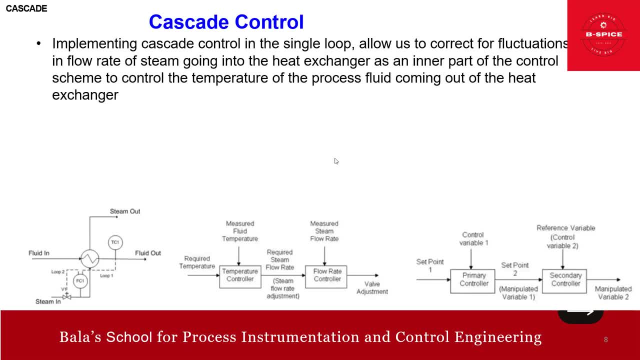 let us see the cascade. i hope you got it right. okay, see, implementing a cascade control in a single loop. allow us to correct for fluctuations in the flow rate of the steam. you got it right. this flow rate of the steam is going to be going into the heat exchanger as a inner part of the control scheme, because you remember this. 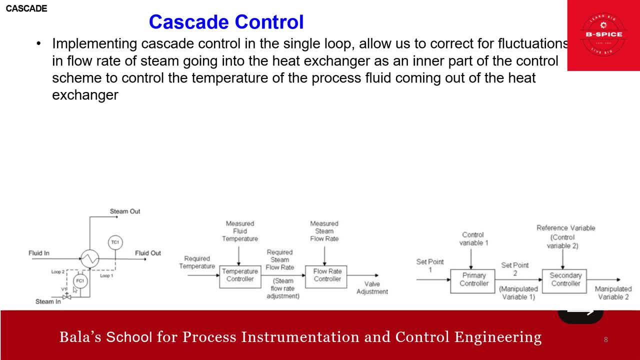 is your primary outer and this is your secondary slave. this is the inner- okay, so inner- part of the control scheme to control the temperature of the process freedom control the temperature of the process fluid coming out of the heat exchanger. i hope you got it. okay, a basic cascade control. 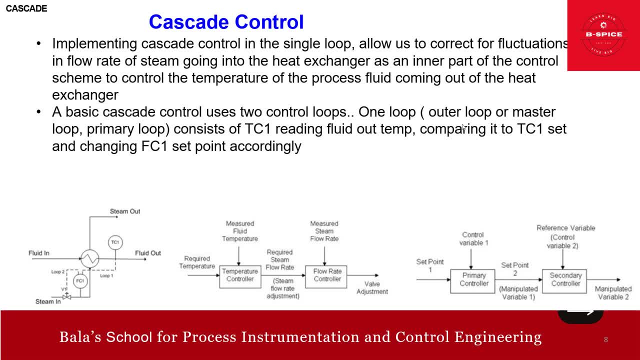 uses two control loops. okay, one outer loop- actually this is outer loop for master, this one okay, or primary. it consists of a pc1 reading the outplot temperature, right outlet temperature and comparing with the set point and changing the fc1 accordingly. you got it, friends. i hope it is. 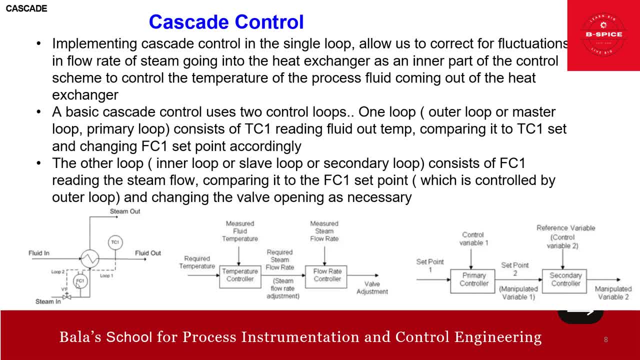 clear. the other one is the inner loper. this one is the inner loop, okay, or slave loop, or secondary loop. consists of fc1: okay, reading the steam flow: okay, and comparing with this set point, which is controlled by the outer loop: okay, because the set point is driven by a sender, ok, and then you play, this will come out: keeping control of the drag, control of the flow guideная. 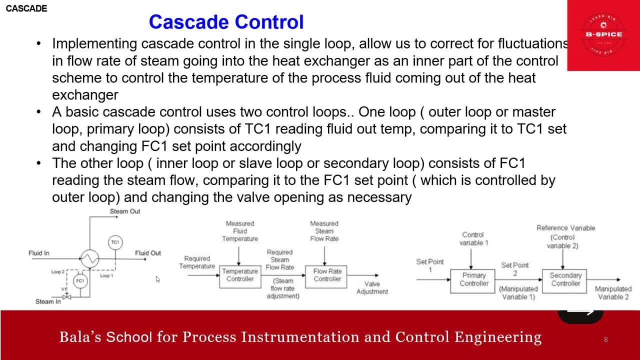 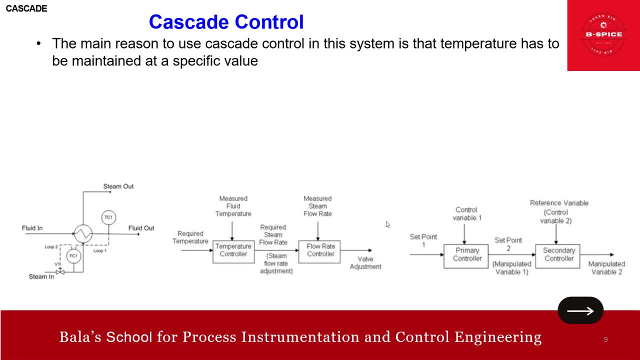 by this f right, yes, and changing the valve opening as necessary. i hope this is also clear. now we are good to go. the basic control have two loops, okay. one is outer loop, other is the inner loop. we are ready, right, okay, good, now i have to add a bit more. see, you may ask what is the main. 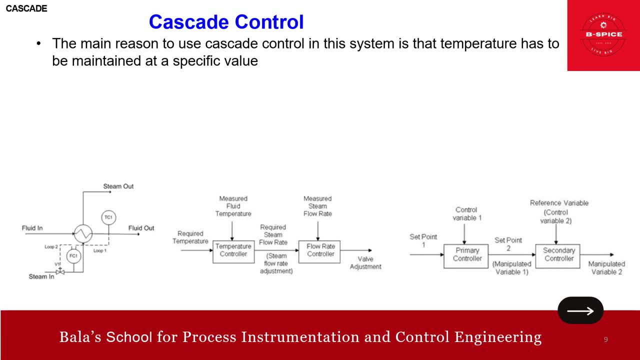 reason, see, the main reason to use cascade control in this system is that the temperature has to be maintained at a specific value. so that is the- you know, our aim actually. so the valve position does not directly affect the temperature. so that is another point. this valve position does not. 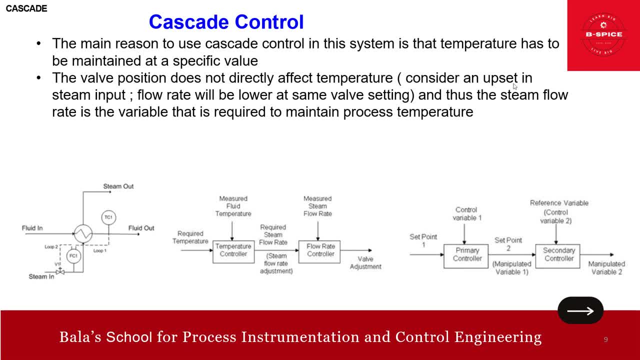 directly affect the temperature. okay, see, for example, consider upset in steam input. okay, the flow rate will be lower than the same valve setting right? yes, and thus the steam flow rate is a variable, that is, the steam flow rate is a variable that is required to maintain the process temperature. okay, you got it right. so the valve position does not. 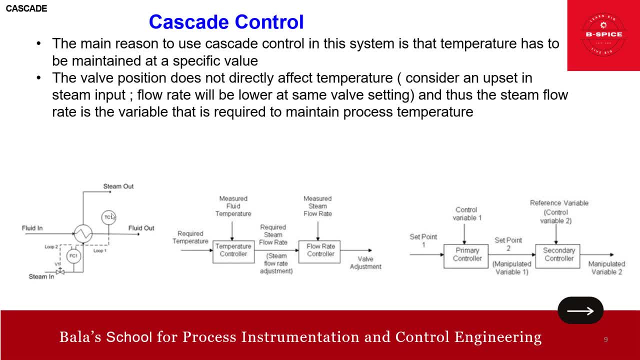 directly affect the temperature. okay, and thus the steam flow is the variable that is required to maintain the temperature. you got it, friends, okay? so because of that, the inner loop is chosen to be the inner loop, because it is prone to higher frequency variation. you know this is. 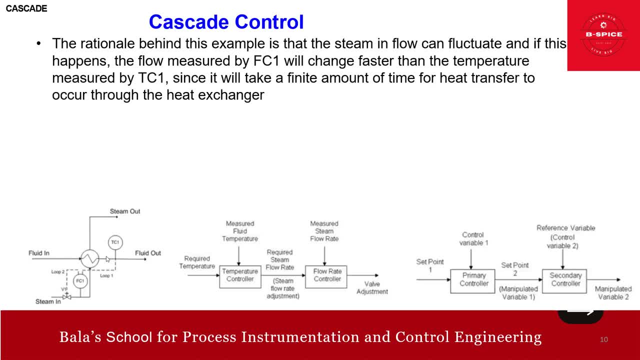 inner loop. okay, right now to add a bit more. the rational behind in this example is that the steam inflow can fluctuate. okay, and if this happens, the flow measured by fc1- okay- will change faster. very important friends, just remind, uh, just focus on it. the rational behind this example is that the steam in the flow can fluctuate. steam inflow. 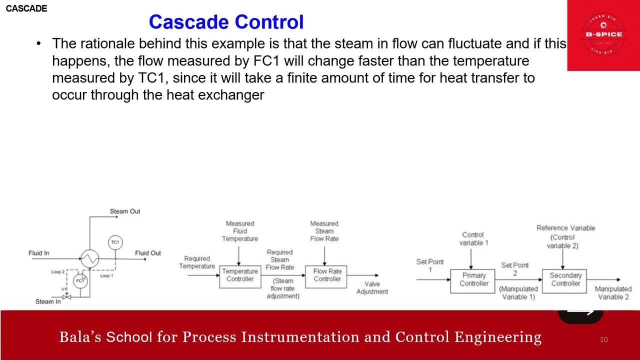 can fluctuate and if this happens, the flow measured by the fc1 will change faster than the temperature measured by the tc1. you got it right, since it will take a finite amount of time for the heat transfer to occur through the heat exchanger. so the point is you have c1 will change then faster. 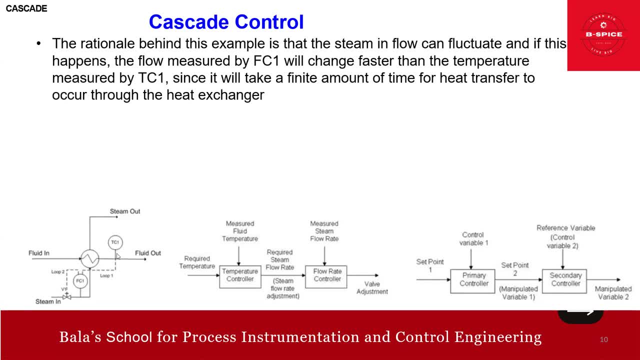 than the temperature tc1, because the tc1 will take a finite time of changeum for heat transfer to occur through the heat exchanger. you got it fine, okay, good, since the steam flow measured will go dreams. so air temperature will go up by the FC1 changes at a higher frequency. Okay, We choose this to be inner loop. Okay, Okay. 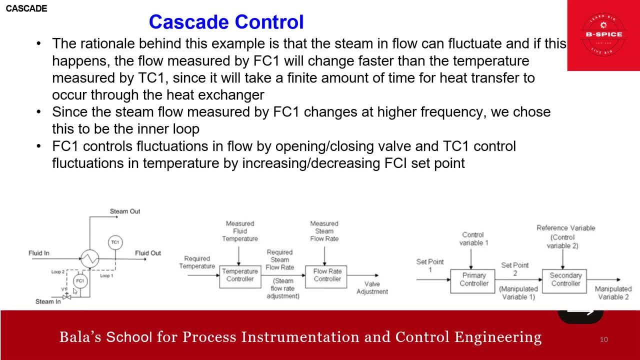 So the FC1 controls the fluctuations by opening or closing the valve and TC1 controls the fluctuations in the temperature by increasing or decreasing this FCI set point. You got it now. I hope it is very clear. Okay, Good, Thus cascade control: use two inputs to control this. 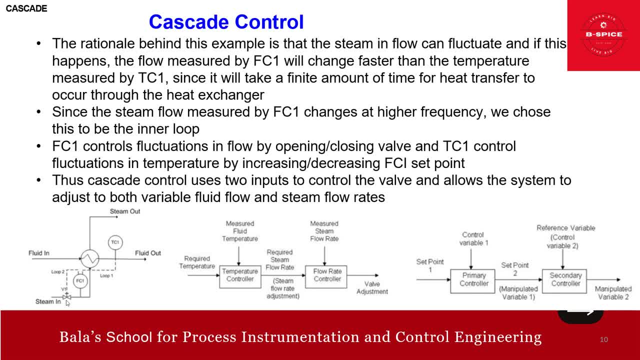 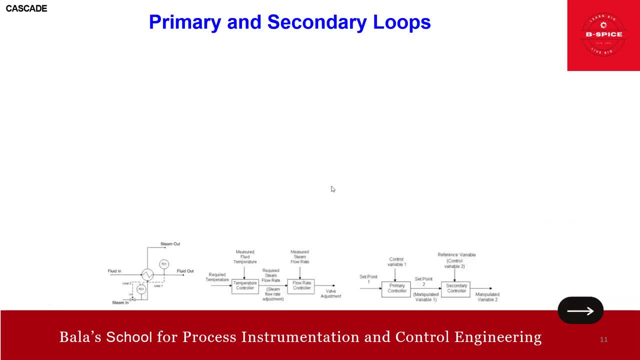 valve, Okay, Allows the system to adjust both variable fluid flow and the steam flow rates. Okay, friends, I hope now it is very clear. Right Now let us see a bit of example of primary, basically an explanation. Okay, As we discussed earlier, loop 1 is a primary. This one, TC1, is. 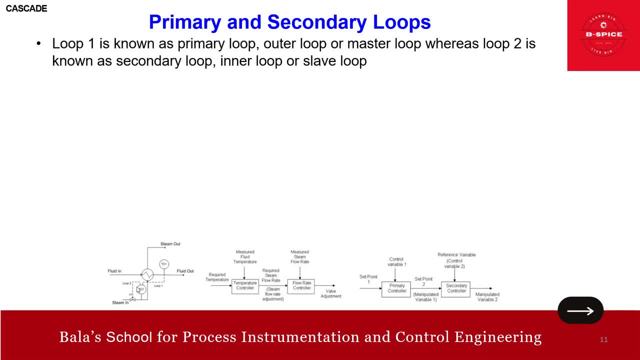 primary- Okay, Outer loop, or master loop, Whereas loop 2 is known as secondary loop, inner loop or sleigh loop. It might be, you know, you may feel like it is repeated, but never mind. See, this is to give a 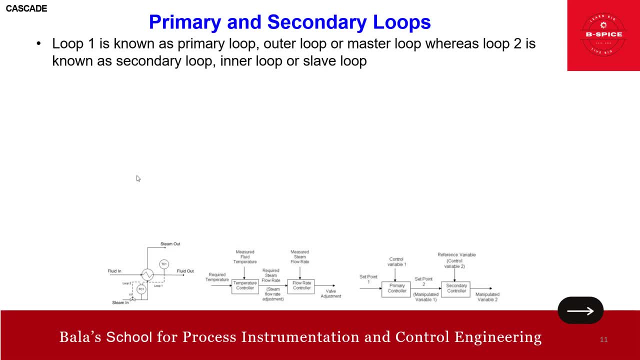 you know better explanation. Okay, In fact, I suggest you have to you know, watch this, you know, couple of times so that you will get the concept very clearly, So that it is very easy for you to you know face the interview or even during your- you know- implementation. All these, 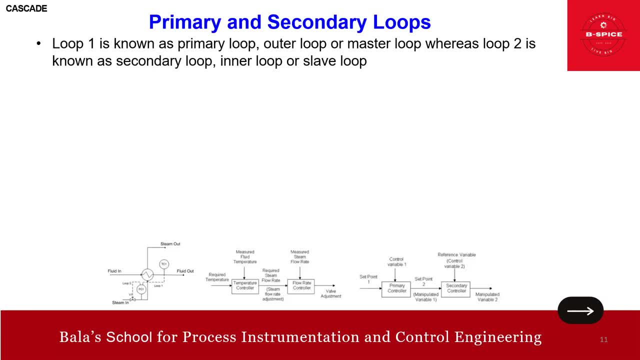 will be helpful And, friends, if you are happy with this concept and if I have explained you know, if you feel that the explanation is good, please, like the friends, Just press your, you know, show your support by pressing the thumbs up button. Okay, Yeah, To identify the primary and the secondary loop. 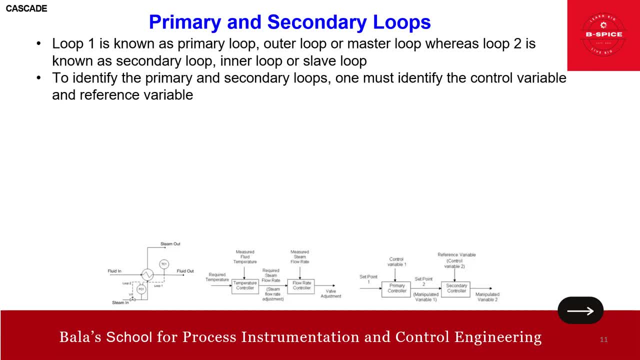 we need to identify the control variable and the reference variable. That is the point How we are, you know, identifying the primary and secondary loop. Yeah, We need to know that: control variable and reference variable. Okay, friends, Okay, As you can see here, this is your control variable. Okay, This is your. 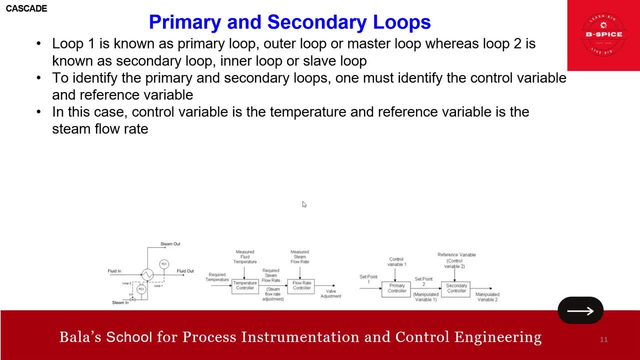 reference variable. So that is how we need to classify. Okay, In this case, you know, control variable is that what Temperature? Right? Reference variable is that steam flow rate? Very easy, Right, Yes, Hence the primary loop one involves control variable and secondary loop two 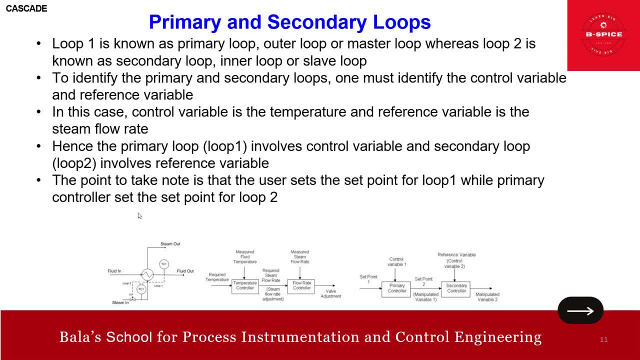 okay, involves the reference variable. Good to go Right. Yes, The point to take note is that user sets the set point for loop one. Very, very important friend, The user, meaning us. we set the set point for loop one and temperature, While the primary controller, this temperature one, set the set. 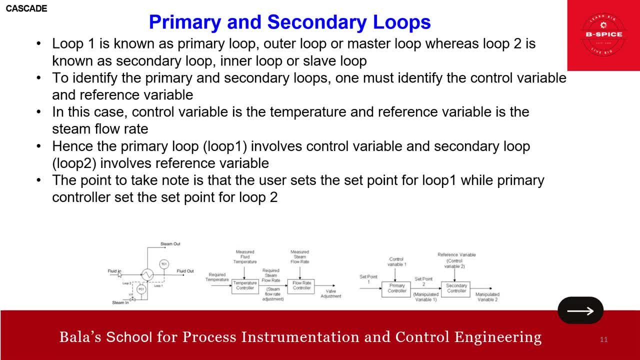 point for the loop two, That is, the flow control. Okay, Got it. So master control responds to slow changes. This master control responds to slow changes, while slave controller responds to fast changes. So this is that, because this is, you know, inner loop. Okay. 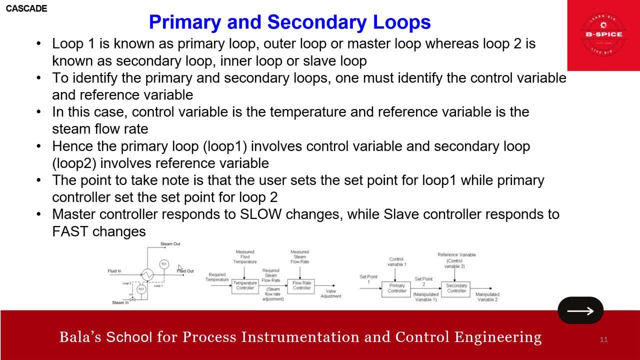 So because of this inner loop, we have an advantage also. We will explain that in the next subsequent slide. Okay, You just remember. master controller responds to slow changes, while slave controller responds to fast changes. Okay, Now, when to use the cascade control. This: 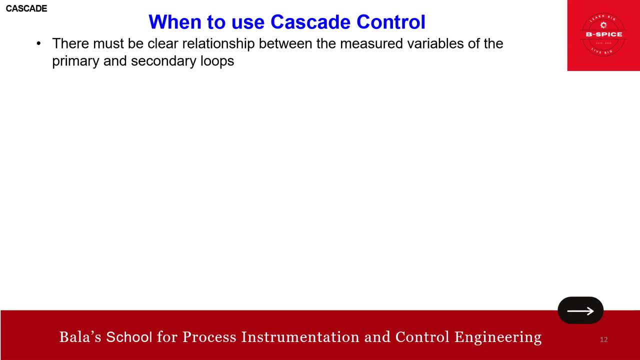 is the question. See, simple friends. There must be clear relationship between the measured variable of the primary and secondary loop. That was a one point, Clear relationship. Okay, Right, The secondary loop must have influence over the primary loop. You got it, friends: The secondary. 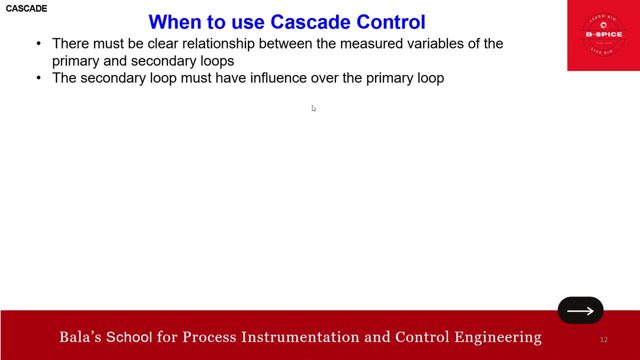 loop in that in our case it was a flow loop right- That must have influence over the primary loop. That's it. So another point, very, very important point: The response period of the primary loop, that is a temperature one, has to be at least four times larger than the response. 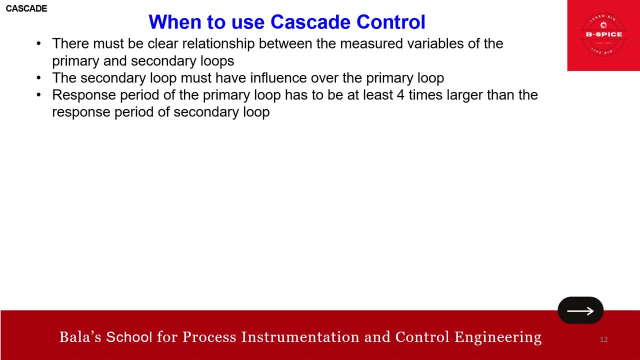 period of secondary loop Very, very, very important. The response period of the primary loop has to be at least four times larger than the response period of the primary loop, So the response period of the secondary loop. Okay, Right, So major disturbance to the system should. 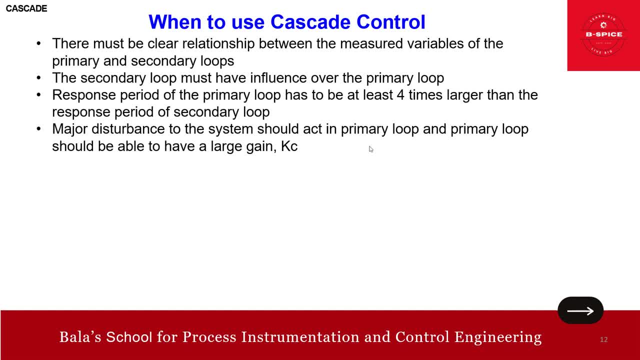 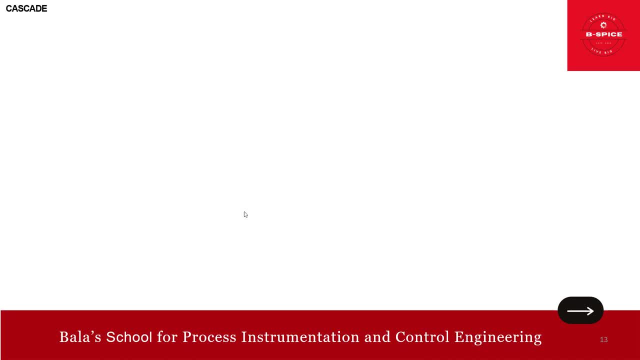 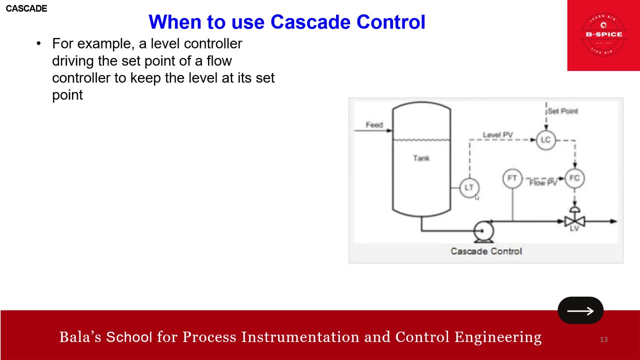 act in the primary loop. So that is the pointer: Major disturbance will act in the primary loop And primary loop should be able to have a large gain. Okay, That is the pointer. So those case we can use this cascade control. Okay, For example, we can see this, You can see here: 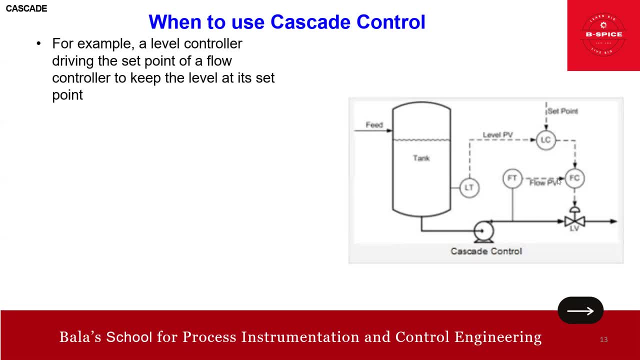 this is a typical cascade with a level controller and the flow controller. Okay, Right. For example, it's driving the set point of the flow controller to keep the level at its set point- Okay. The flow controller, in turn, drives the control valve. Okay, To match the flow. To match the flow. Okay With. 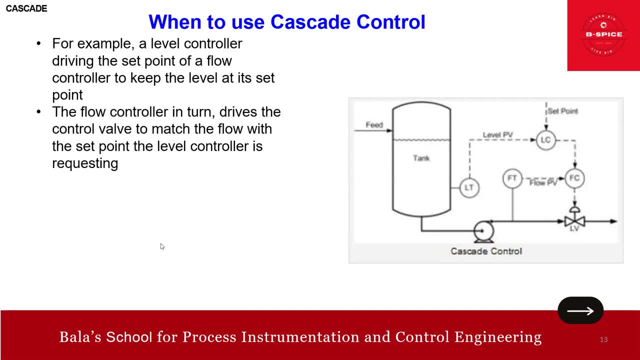 the set point of set point, the level control is requesting. Okay, You got it Right. So there are several advantages of cascade control. Most of them is to isolate the slow control loop from non-linearities in the final element. Okay, So that is the point. Okay, So that is the point. Okay So. 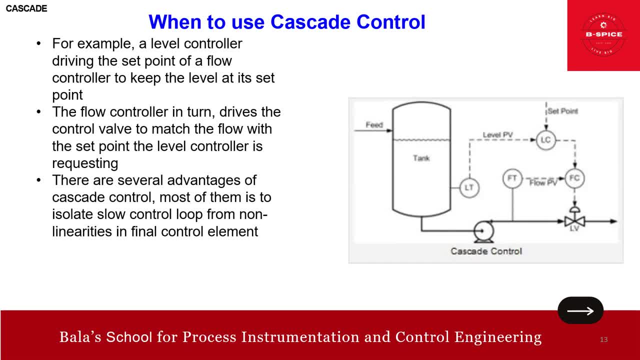 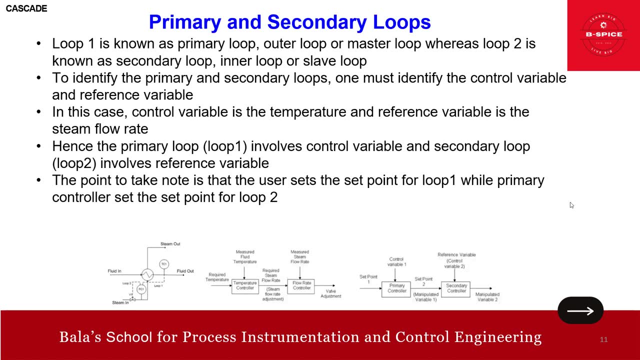 that is the important pointer. Okay, To isolate the slow control loop from non-linearities in the final control element, As you can see here. maybe I go back again to refresh your memory. Yeah, You see, master controller responds to slow changes, Slave controller responds to fast. 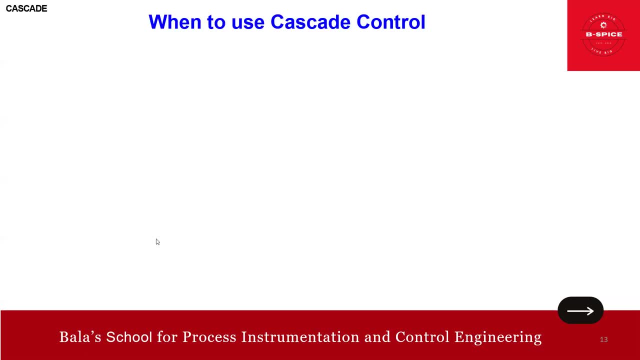 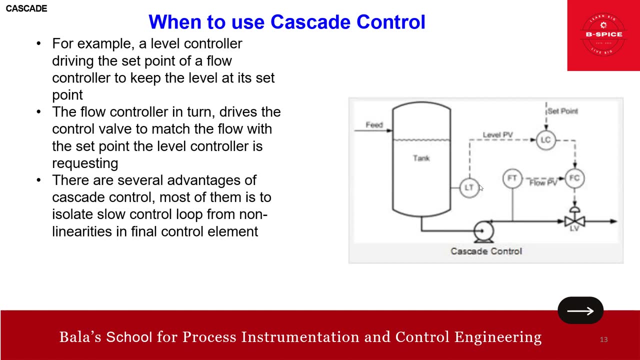 changes, Right, Yes. So here coming back, so to isolate the slow loop from the non-linearities. So here, what is the slow loop? This is the slow loop, Right, Yes, This is your final control element. I mean, this is your. 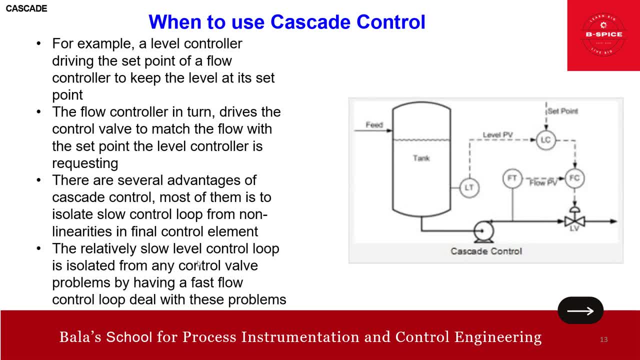 inner loop which is faster Right. Yes, So the relatively slow control loop is isolated from any controller problem by having the fast flow control loop dealing with this problem. So who is this fast flow loop? Here is the flow. is the fast flow loop dealing with this, all this problem? 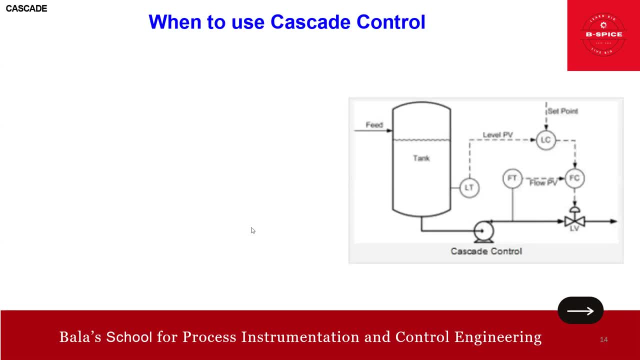 You got it Right, Okay, Good. So when to use the cascade control? The same thing. Imagine that the control was, as a stick problem, a stickion problem. Okay, So without the flow control loop, this, the level control loop driving this valve, the sticky valve will continuously oscillate in a 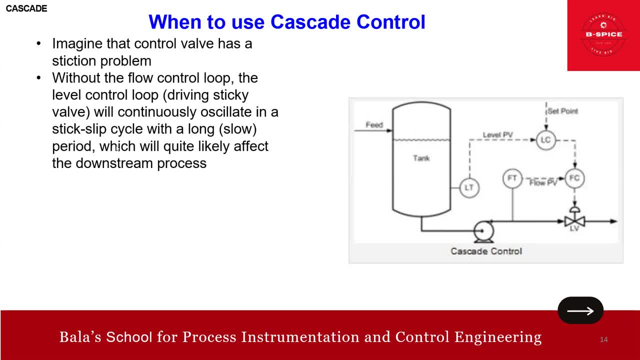 stick slip cycle with a long slow period, which will quite likely affect the downstream of the process. You got it, friends: If we do not have them, okay, flow control loop, Okay, Then this control valve is having a sticky issue, actually. So 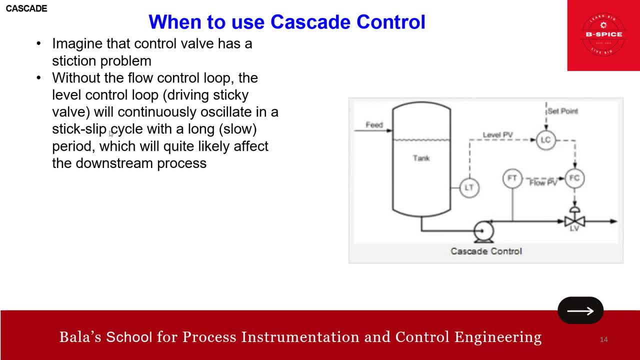 if we only control using this level, then it will actually, you know, oscillate in a slip cycle, with a long slow period, which will quite affect, likely affect, the downstream process. So that is the point. So if the fast flow control is in place, fast flow control is in place. 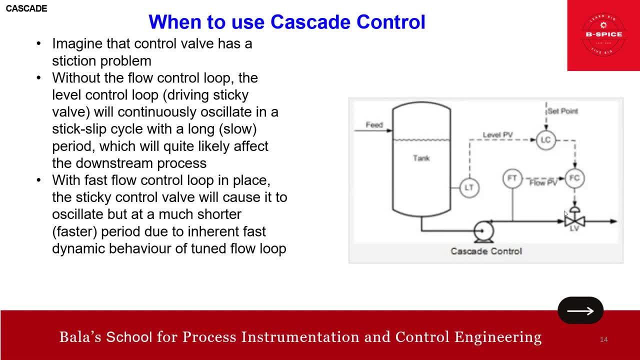 the sticky control valve will cause it to oscillate. Oscillation. oscillation will be there, but at a much shorter rate. So, due to inherent fast response of this dynamical behavior of the flow tuned loop. Okay, friends, I hope you got it. So, basically, 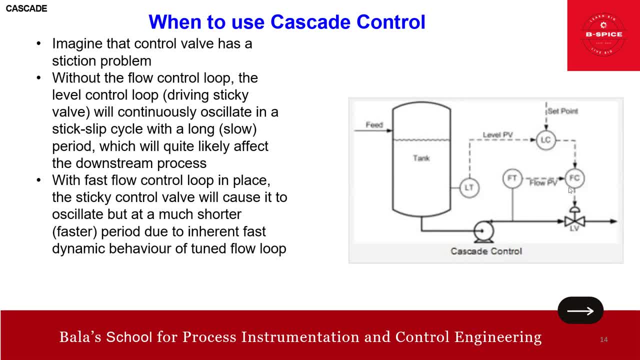 whatever is the problem here, that will be, you know, taken care by this inner loop, So it will not have a direct impact because of the slowness of the outer loop. Okay, You got it right. So it is likely that fast oscillations will be attenuated by. 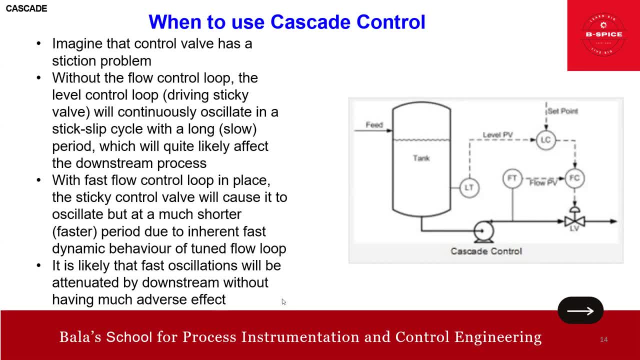 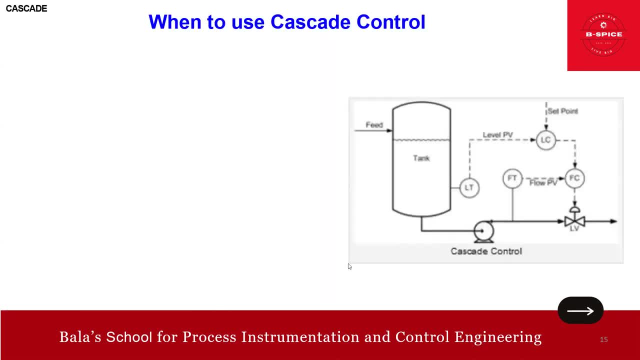 by downstream without having much adverse effect. It is likely that fast oscillations will be attenuated by downstream without much adverse effect. Okay, So to add on more, another problem: imagine that the control has a nonlinear characteristics. This one, nonlinear. 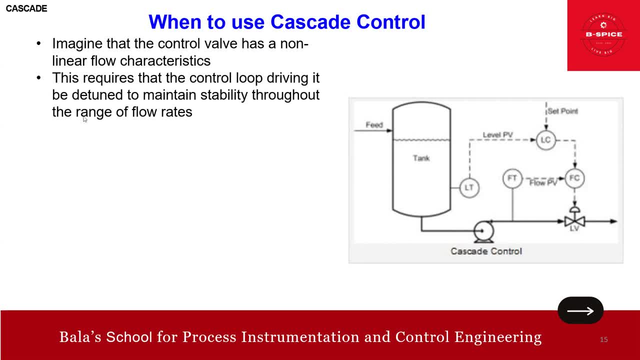 characteristics. Okay, This requires the control loop driving it to be detuned to maintain the stability throughout the range of flow rate. So if the level controller directly drives the valve, directly drives the flow rate, then it will not have much adverse effect. So if the level controller 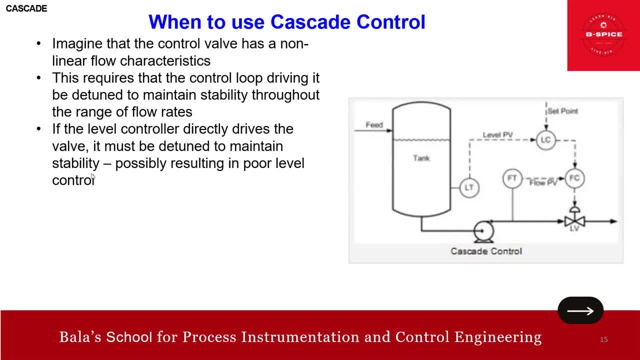 directly drives the valve, then it will not have much adverse effect. So if the level controller directly drives the valve, it must be detuned to maintain the stability. possibly it will result in a poor level control. So in cascade control arrangement with flow control in place of 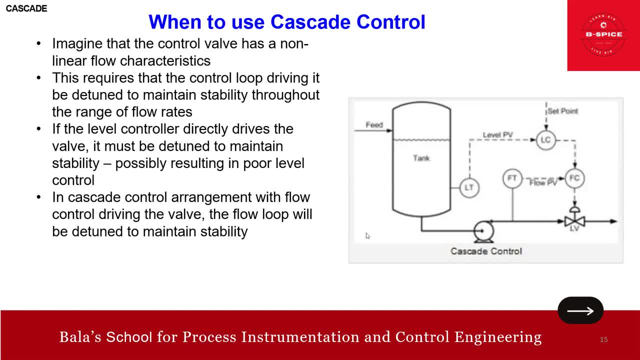 driving the valve, the flow loop will be detuned to maintain the stability. Okay, So the result is relatively poor flow control. but as the flow is dynamic, dynamically, so much faster than the- you know- level loop, this level loop control is hardly affected, So it will not have. 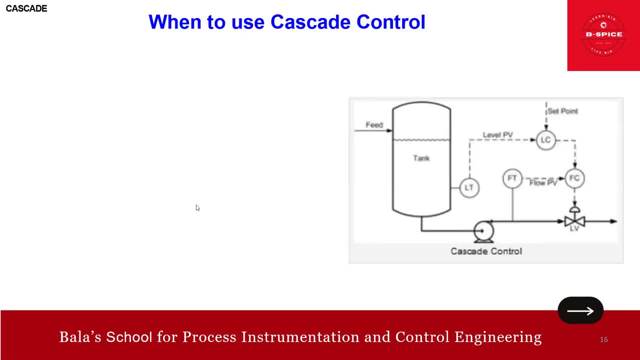 any impact on the level loop. So that is the point. Okay, In cascade architecture, okay, the inner, inner secondary, inner secondary: this one serves as an early warning process variable and the essential design characteristics for selecting PV to include: see, basically, it should be: 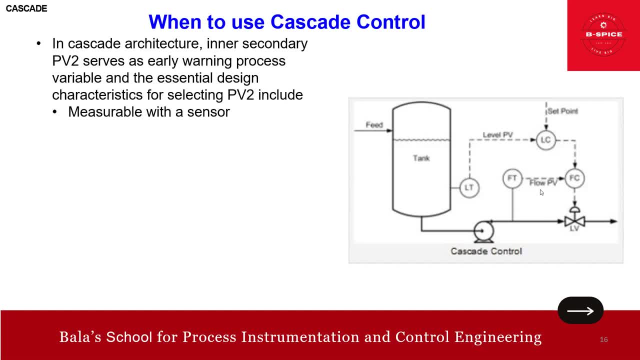 measurable. I do not know whether you are following, friend. See, what I am trying to explain is, in this architecture, inner secondary loop, which is the flow loop, it serves as an early warning, meaning it detects actually any problem. is there? 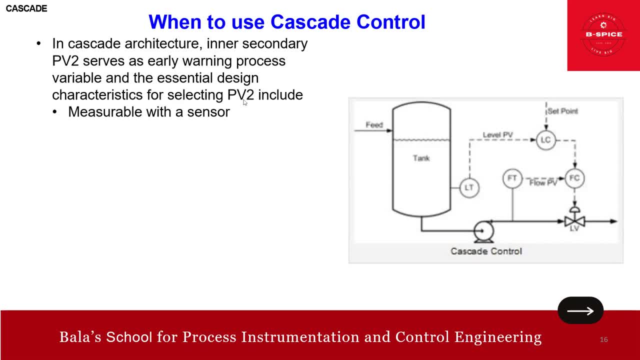 it detects early actually. And the essential design characteristics for selecting- see what are all the characteristics for selecting this PV2?? So it should be measurable with a sensor. So here we have a flow transmitter, so it is measurable with a sensor. 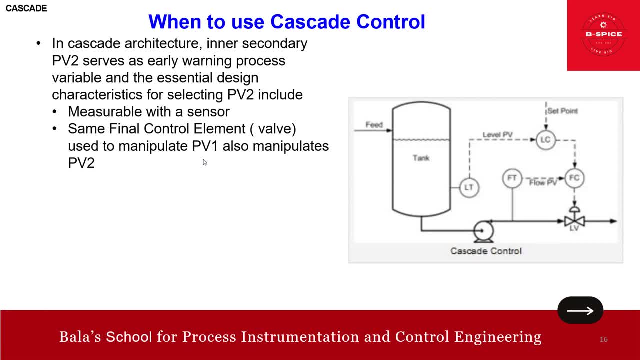 Got it right. Yes, It is the same final controlled element used to manipulate PV1,. also manipulate that PV2.. These are the scenarios, conditions actually requirements: the same final controlled element. okay, well, used to manipulate PV1,. okay, and PV2,. 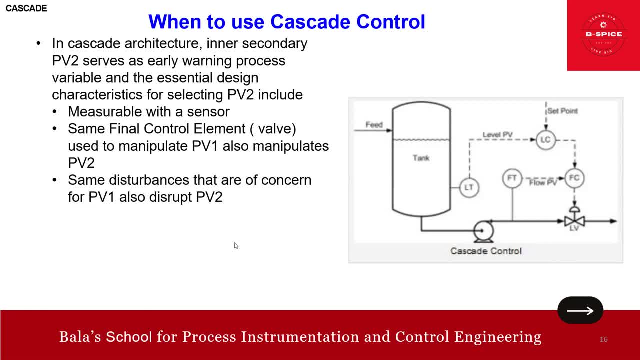 also manipulates PV2.. That is the point. Same disturbances that are of a concern for PV1 also disturb the PV2.. PV2 responds this one responds before PV1 to disturbance, the concern and to final controlled element manipulation. So this actually flow actually responds before PV1 to 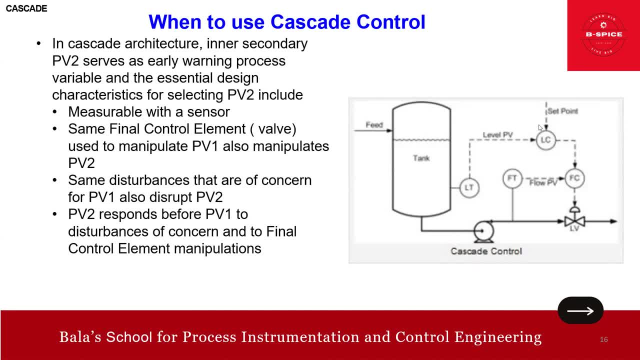 disturbance of concern. So this is the point. So this is the point. So this is the point. So if any disturbance occurs before any disturbance occurs here, so this gentleman here, the PV2, will respond. actually, right, So that is the point. All these should be there. This is just part of 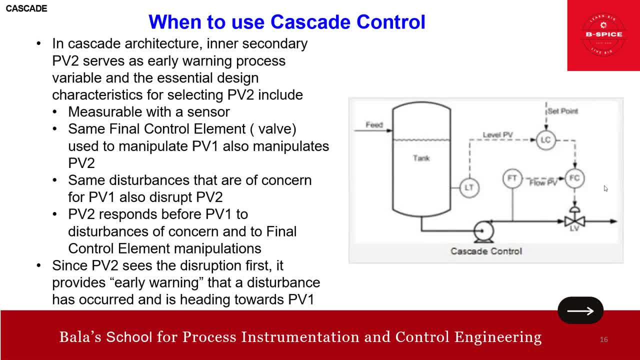 the characteristics. actually, Since PV2 sees the destruction first, he sees the destruction first, it provides the early warning that a disturbance has occurred and is heading towards the PV1,. okay, That is the point right. So to add on: 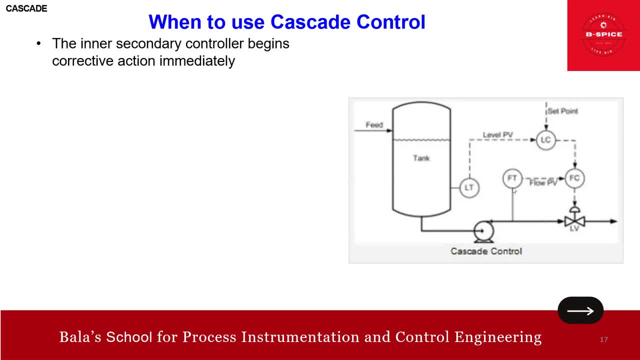 the inner secondary controller begins corrective action immediately. This will actually do the corrective action immediately, Since PV2 responds first to the final controlled element. since the PV2 responds first to the final controlled element, manipulation, disturbance rejection can be well underway even before primary variable has been substantially impacted by the disturbance. So 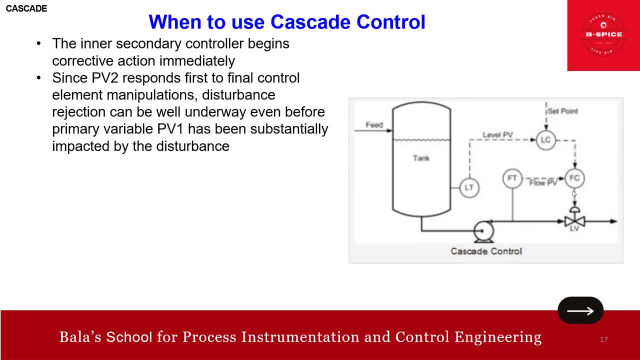 that is the point, Since this immediately actually response to the final controlled element- manipulation, disturbance rejection- can be well underway even before primary value has been substantially impacted by the disturbance. okay, So in cascade control of the primary process, variable PV1 will benefit by corrective. 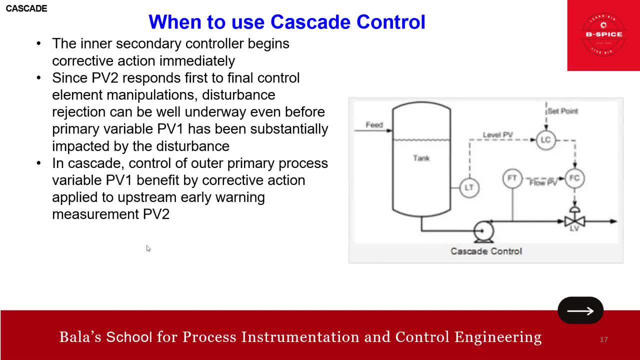 action applied to the upstream early warning measurement of PV2.. So this is just only explaining and repeating. actually, In a cascade control, control of the primary value has been primary process, primary process, variable benefit. actually okay, how, by corrective action, apply to. 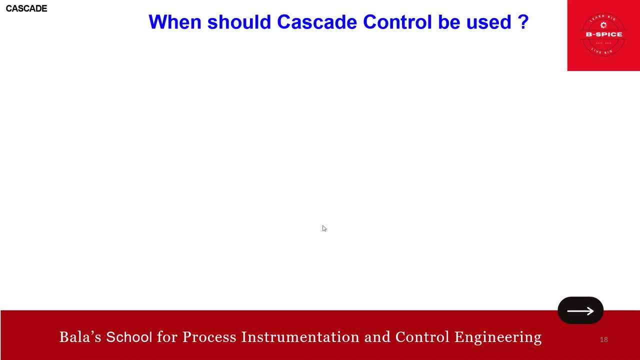 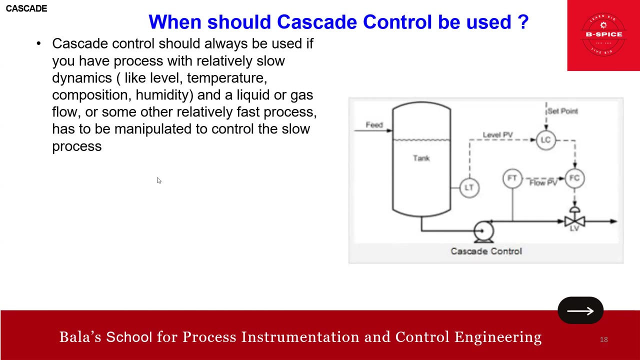 the early warning of the measurement PV2,. okay, friends, okay, So we have seen. now, when has to this what you call cascade used? Now, when should cascade? it is a condition, actually it is a must. okay, cascade control always be used if you have the process with a relatively slow, dynamic sense. 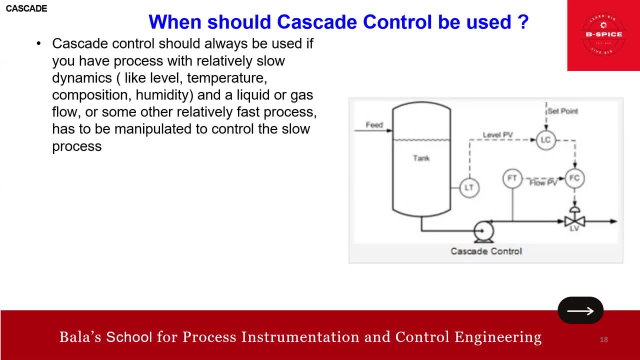 slow, dynamic in the sense of level, temperature, composition, humidity, all these and a liquid or gas flow or some other relatively fast process has to be manipulated to control the slow process. So these are the scenario we should use. the cascade control always be used if you have a. 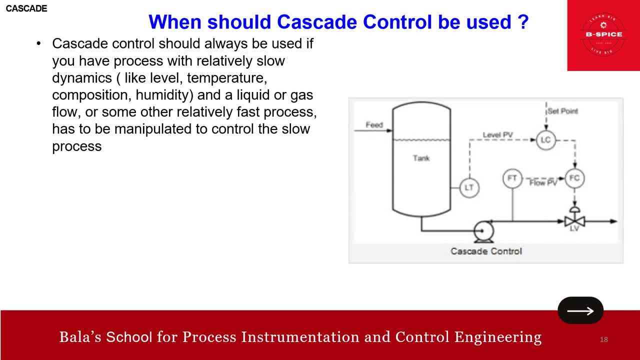 process with relatively slow dynamics in the sense level, temperature, composition or humidity. all these and a liquid or gas flow or some other relatively fast process has to be manipulated to control the slow process. That's a point. For example, changing the cooling. 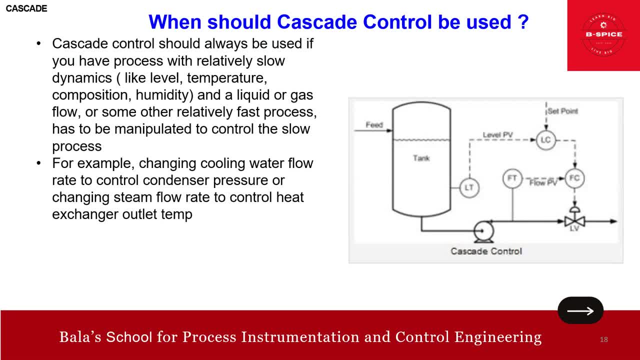 water flow rate to control the condenser pressure, or changing the steam flow rate to heat up that heat exchanger out rate temperature. These are the typical example of changing the cooling water flow what for to control the condenser pressure or changing the flow rate to control heat exchanger. 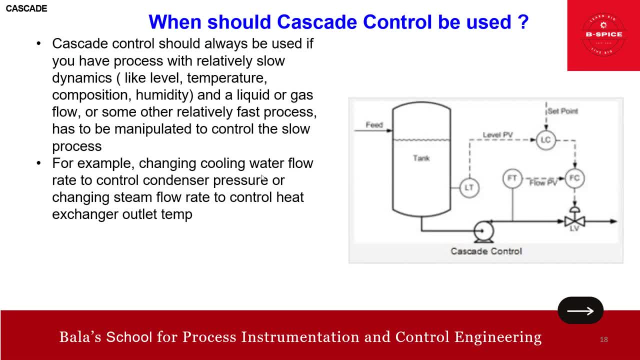 temperature. As you can see here, friends, you have two elements right: Control elements, right? Yeah, that is the thing. Yes, So in both cases, flow control loop should be as used as a inner loop in cascade arrangement. Okay, friends, So now we know when. 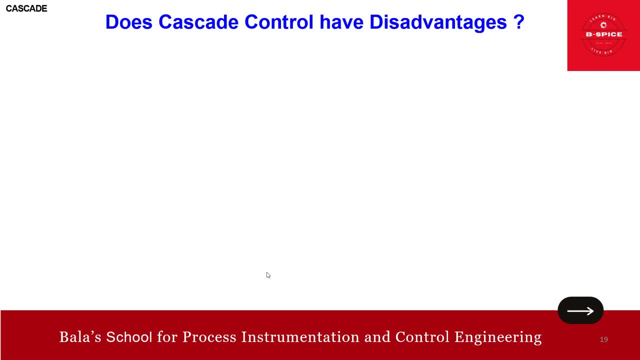 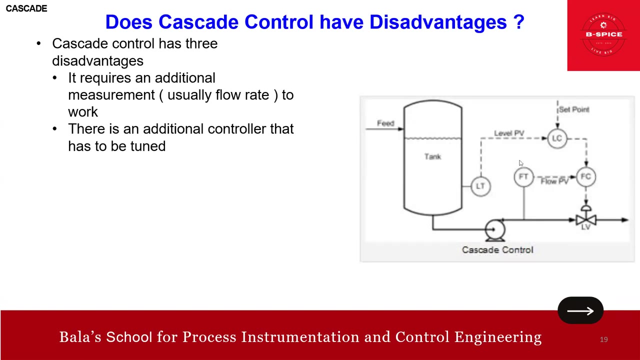 to use the cascade control. Now you may have a question: Does cascade control have disadvantages? Yes, it has. What are those? It requires an additional measurement, usually flow rate up to work. There is an additional controller that has to be tuned. One more controller, right. 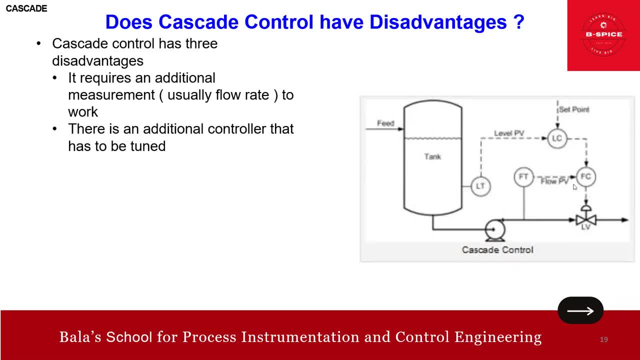 Instead of in addition to this flow, sorry, in addition to this level primary, we have one more. That is a pointer. The control strategy is a bit more complex. That's the point actually. These are the things advantageous, Of course, if we know and if we have a better experience, then not a big. 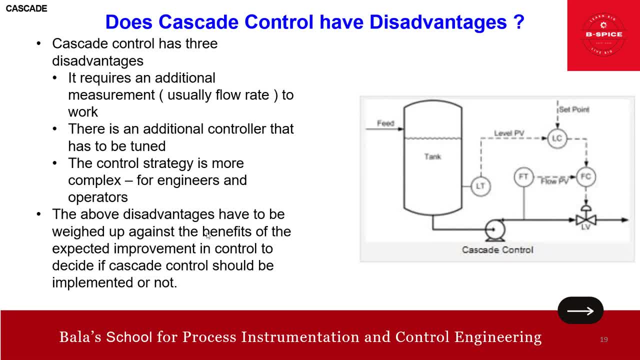 chance but think: but yeah, these are the things that we can say as a disadvantage. The above disadvantages have to be weighed up against them Benefit of the expected improvement. So that is a pointer in control. If we decide, cascade control should be implemented. 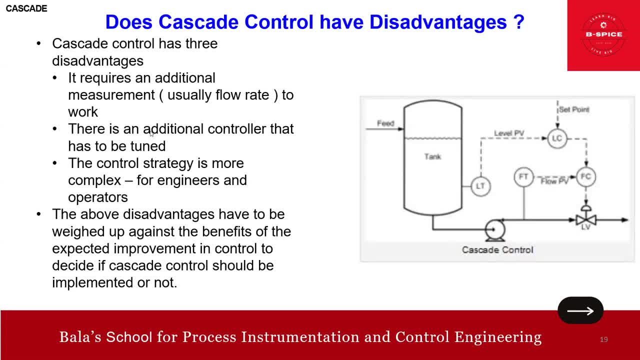 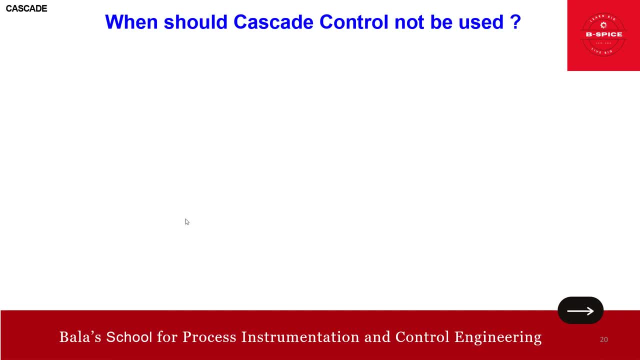 or not. we need to see the benefit. actually, If we have a benefit, then this, all this, will not be a disadvantage. Okay, friends Got it. Okay, good to go Now. when should cascade control not be used? Okay, Cascade control is beneficial only if the dynamics of the inner loop are fast. 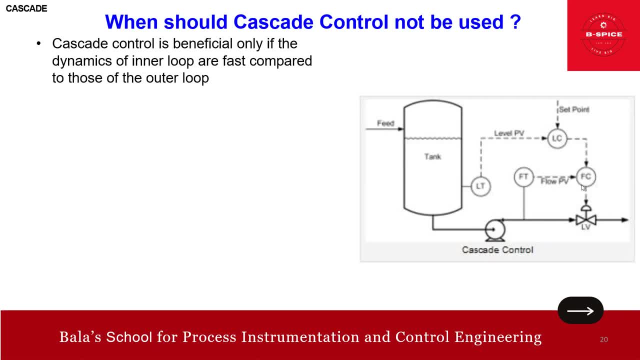 compared to the outer loop. That is the pointer. This: dynamics has to be fast. Okay, that is the pointer. So cascade control should not be used if the inner loop is not at least three times faster than the outer loop. This is a bit confusing, but just listen, friend. 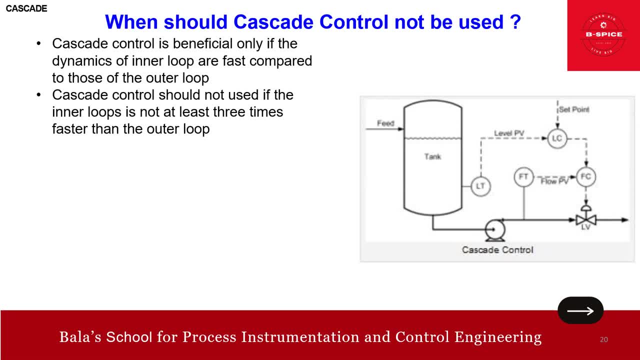 Cascade control should not be used if the inner loop- inner loop, okay- is not at least three times faster than the outer loop, Not at least three times faster than the outer loop. So basically, it has to be Faster. Okay, Got it At least three times faster. Okay, right. So as a rough estimate, 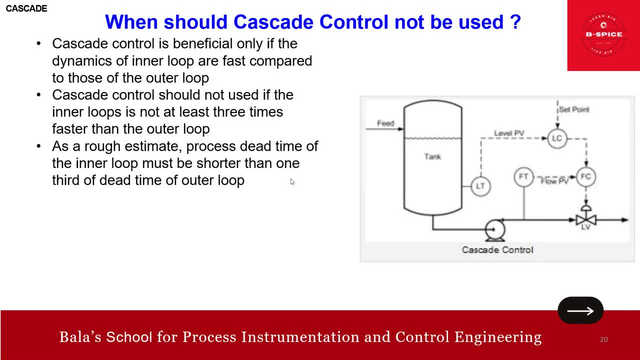 process dead time of the inner loop must be shorter than the third one-third of the dead time of the outer loop. As a rough estimate, process dead time of the inner loop must be shorter than the one-third of the outer loop. So the dead time Okay, Right. So in addition, 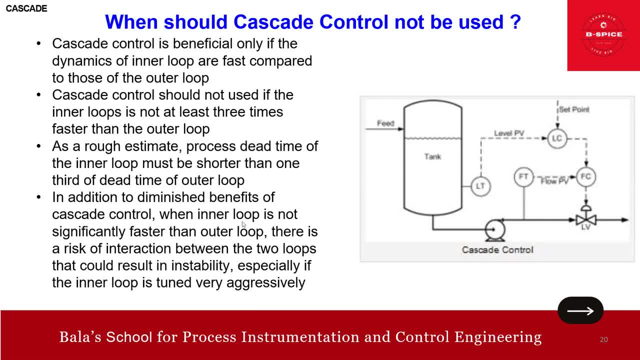 to the diminished benefits of the cascade control, when inner loop is not significantly faster than the outer loop, then the cascade control should not be used. So, in addition to the diminished benefits of the cascade control, when inner loop is not significantly faster than the 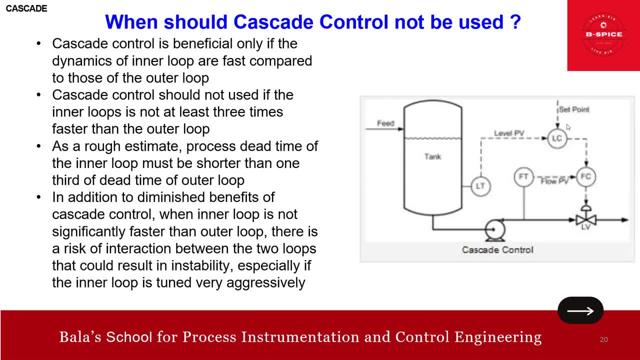 outer loop. when this is not significantly faster than this, there is a risk between the loop that could result in instability, especially if the inner loop is very tuned aggressively. Okay, That point also. you keep it. See, the point is, friend, this has to be faster. Very simple, That's it. 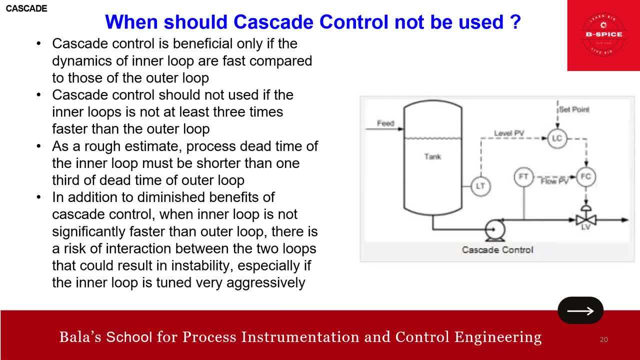 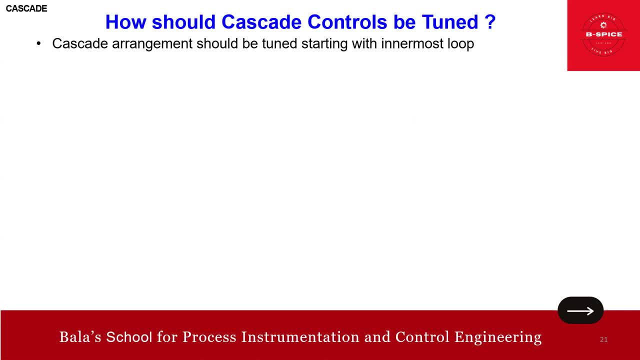 Okay, Okay. Then finally, we will see how the tuning friends. Okay See, basically, I want to, you know, give you a live example. Let's see like it all depends on you know how you are going to support. So if your 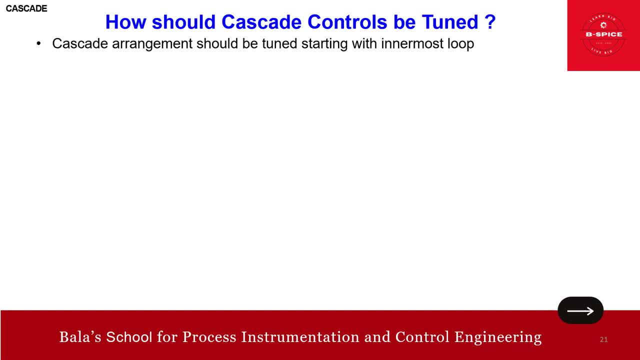 support is better. and if I have a, you know, more subscriber and more watching time, then you know the channel will grow. Then I can even- you know, purchase this, you know this. what do you call the software, the Yokogawa system or any other system? then I can show you the live actually. 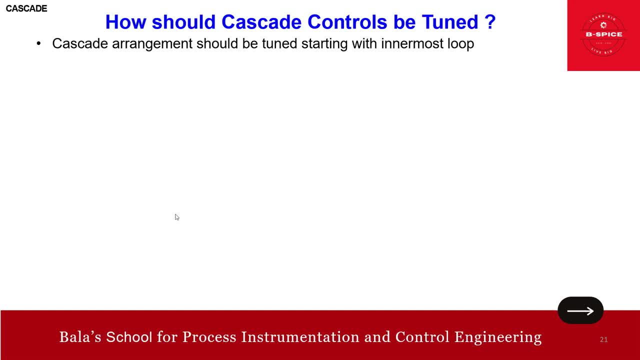 But now, for the time being, bear with me, I'm going to give you some overall idea. Okay, Cascade arrangement should be tuned, starting with the inner loop. Okay, You know inner outer right, So we have to start with the inner loop. So in our case- earlier example- 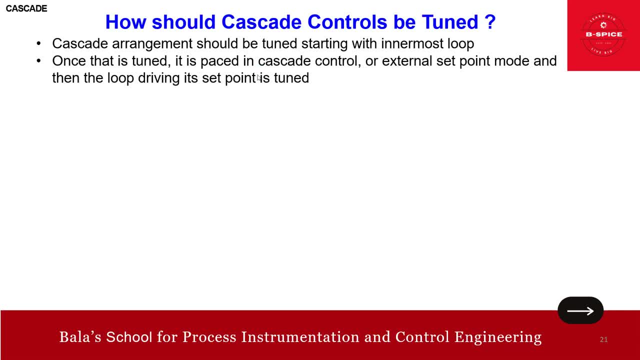 flow loop: Okay. So once that is tuned it is paced in the paced. paced in the cascade control. Okay, Placed, I think, paced placed in the cascade control or external set point mode loop driving is set, point is tuned. So first we need to start tuning the inner loop. 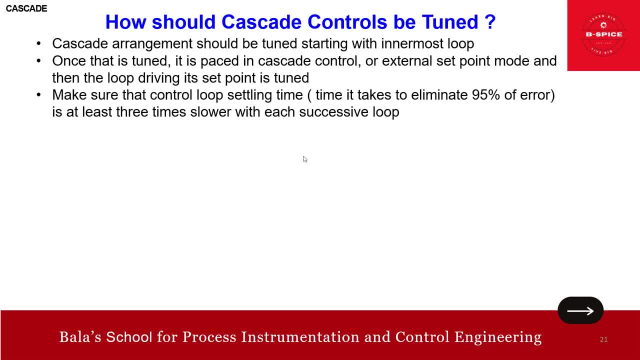 That is the flow in our case and it has to be placed in the cascade loop. Make sure that the control settling time. what is the settling time? This is the time take to eliminate 95% of the error You might have studied during your college days, right? Yes, It applies at least three times. 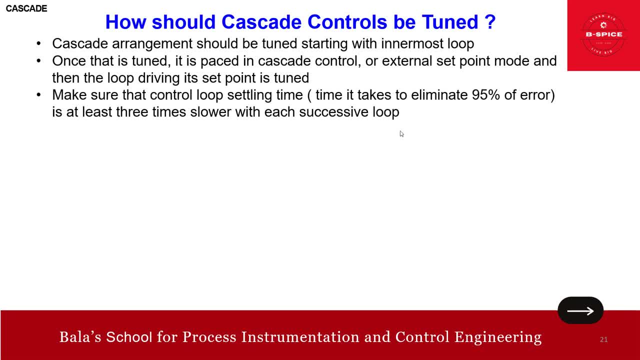 slower than the each successive loop. This point we need to keep take note of. Make sure that control loop settling time is at least three times slower than the each successive loop. If this is not the case, okay, the benefit of cascade control is minimum and it should be questioned. Okay, Cascade system needs. 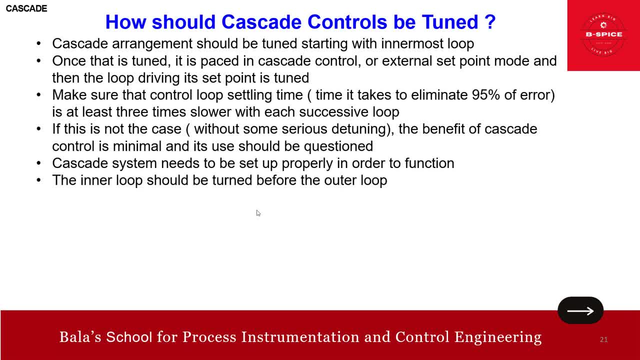 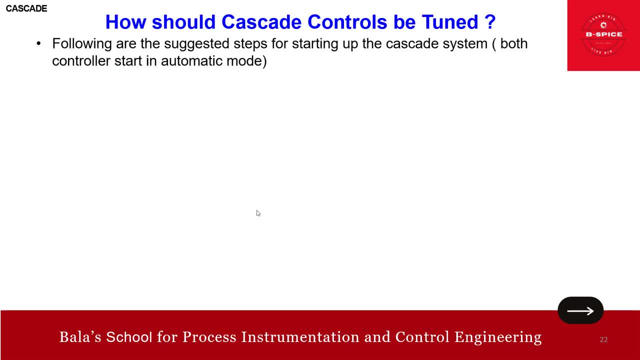 to be set up properly in order to function. Of course, the inner loop should be tuned before the outer loop. Okay, Now we will see the step set. Okay, So, following on the suggested step for starting of the cascade system, both controllers start in automatic mode. Okay, 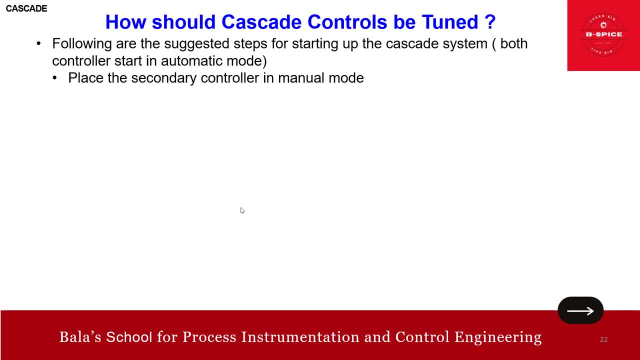 First, we need to place the secondary control in manual mode. Secondary control- What is that? In our case, it is a flow, right? We need to keep that in a manual mode. Okay, If you keep that in manual mode, this will break the cascade and isolate the secondary controller, right. 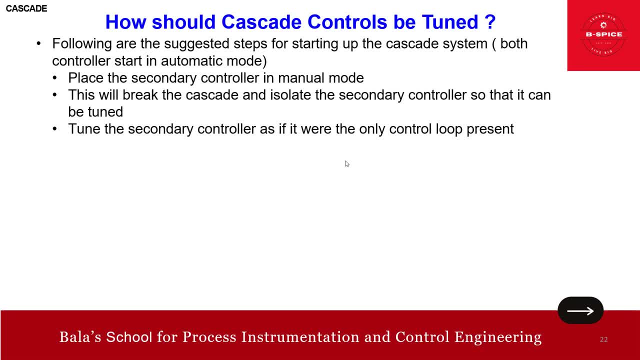 So that it can be tuned. Okay, Now we have taken the secondary controller in manual mode and we start tuning, Okay, Okay, So now when we are tuning, we should think that it's only one control loop is present, because you know, you have taken out right. Yes, 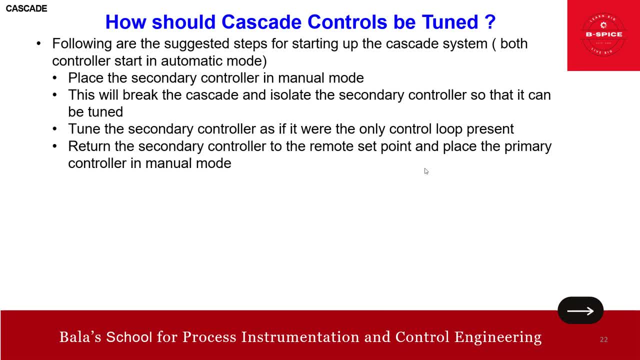 So return the secondary controller to the remote set point and place the primary controller in manual mode. Now we have to return this secondary controller- Okay- To the remote set point And we have to take this primary, which is that? what do you call that? 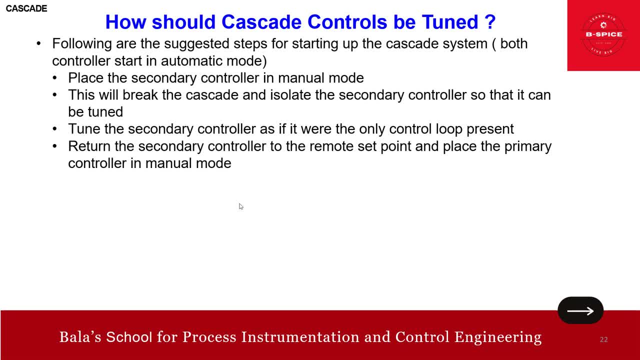 In our example. what is that Flow level? right, Yeah, So the level we need to take in the manual mode. Then, if we do this, then this will isolate the primary controller so that we can tune it. So now we need to tune the primary controller loop by manipulating the set point to the secondary controller. Okay, 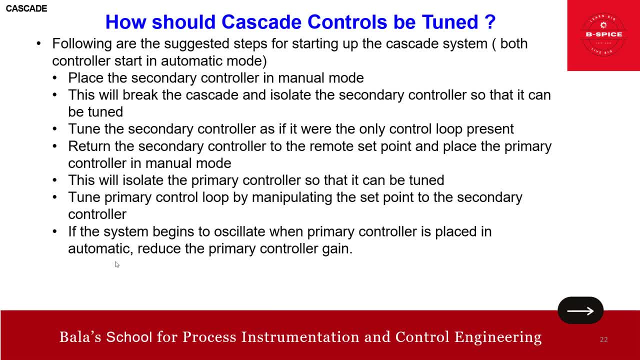 If the system begins to oscillate when primary controller is placed in automatic after we tune we place this primary in automatic right So that time if there is any oscillation, you have to see that we have to reduce the primary controller gain. 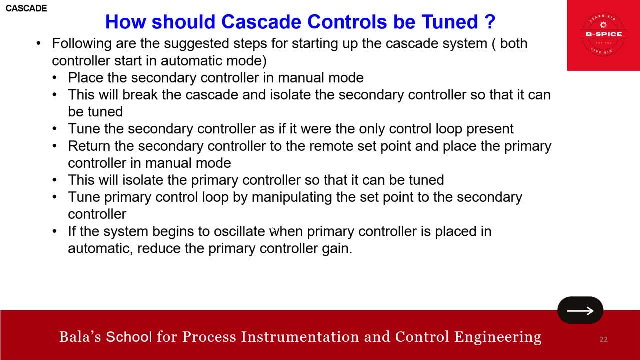 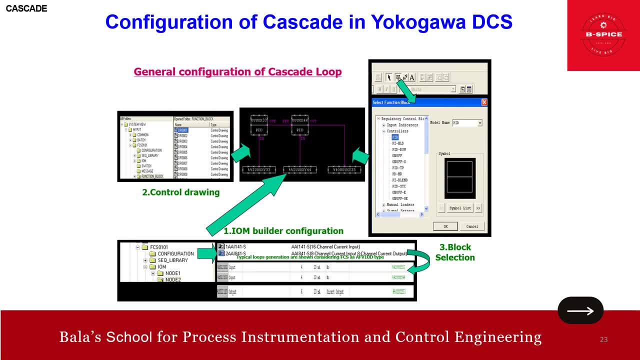 So that's it, friends. That's how we need to do this cascade control tuning. Okay, Now we'll see a configuration: how we are doing the configuration of cascade control in DCS Yokogawa, DCS Friends, if you go to the project builder. 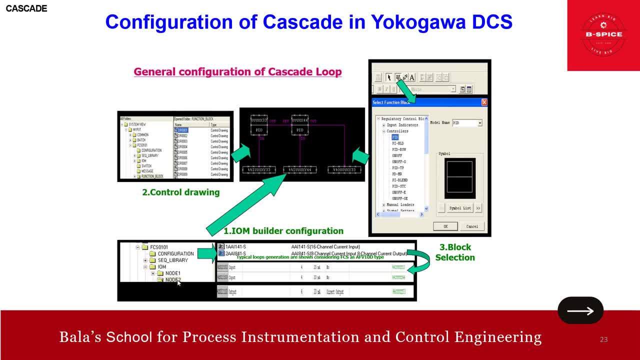 project hierarchy. you can see this node Under this. we have this input right. See, you have two input right And one output Okay. So you have to configure this, Okay, Then after that you have to go to the function block. 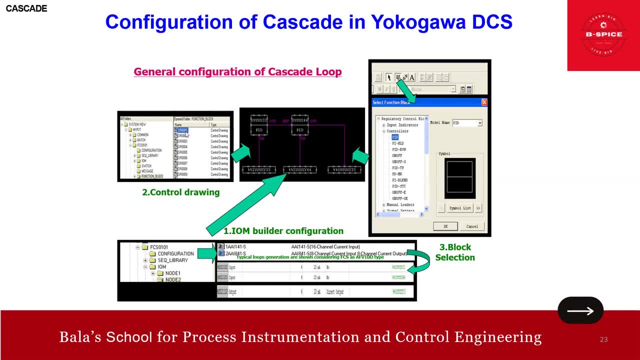 Then under that you have to see the drawing. whichever drawing you are going to configure, When you click the drawing, you will get this. Then, when you press this, you will get all your loop. Then you can see the cascade here. Okay, 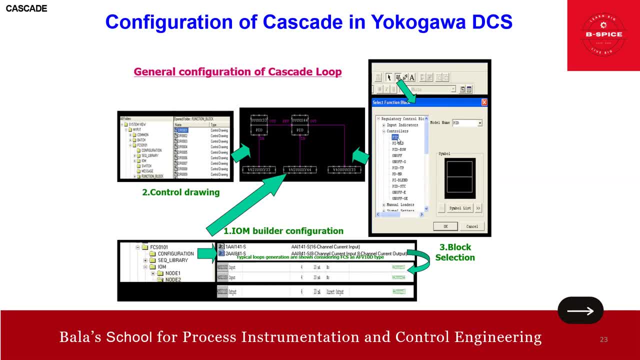 See the PID. Sorry, not PID, Not cascade, actually PID, right? Yeah, because we are using the cascade control, using the PID. So you take the PID, then you drag and drop, As you can see here. this is your input, This is your input, right? Two input. 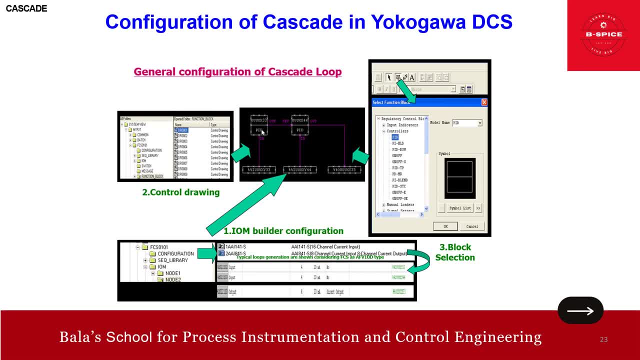 So this is your one controller. This is your what you call primary controller. This is your secondary controller. So this is your in. So the output of the primary controller is going as a set point of the secondary controller. 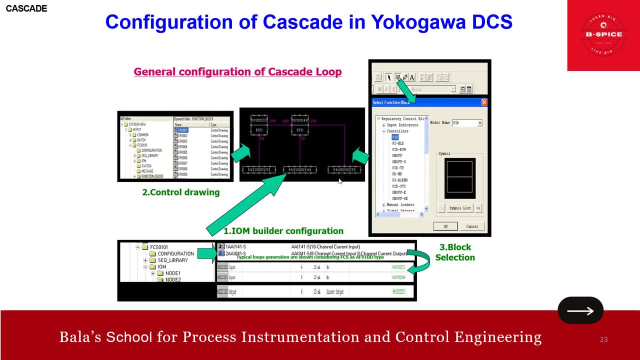 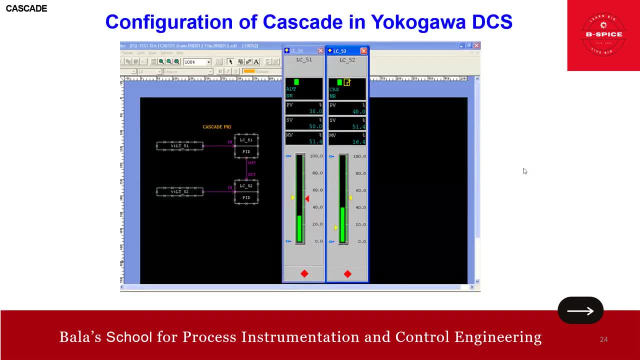 Okay, Out is driving the final control element. You got it, friends. Excellent, That's it, friends, Very simple friends. Okay, Right Now we will see what is another typical example You can see here. this is your cascade PID.